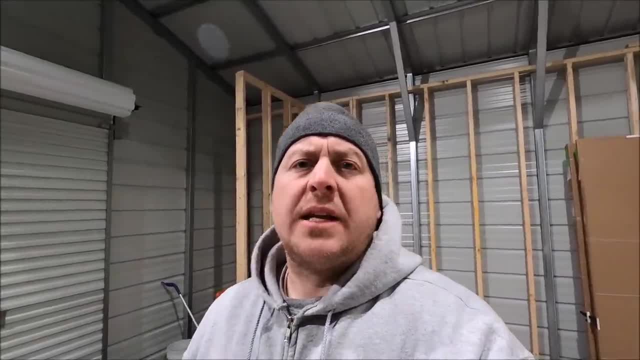 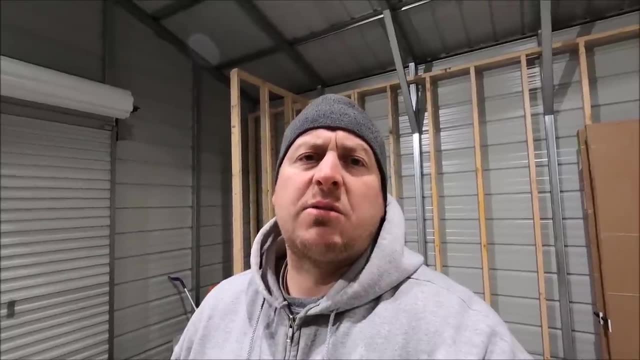 after I get these beams built in the next video, and so I thought I'd take this opportunity just to kind of explain how the wiring is going to go, the wiring process, how three-way switches work, how to wire up outlets, which wire to use, which breakers to use, and just kind of give an overview. 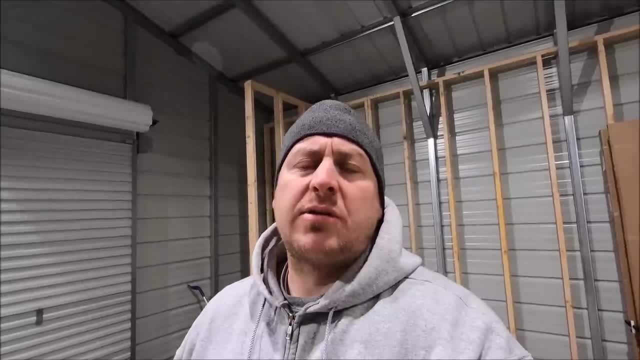 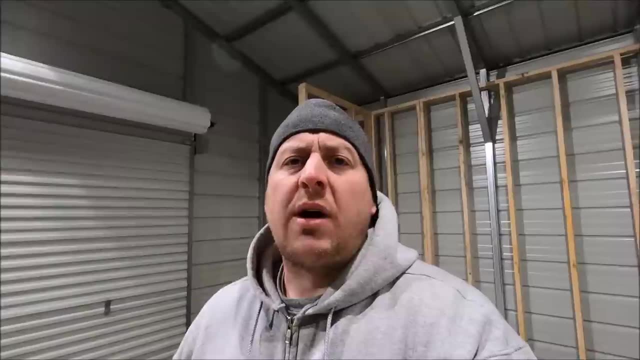 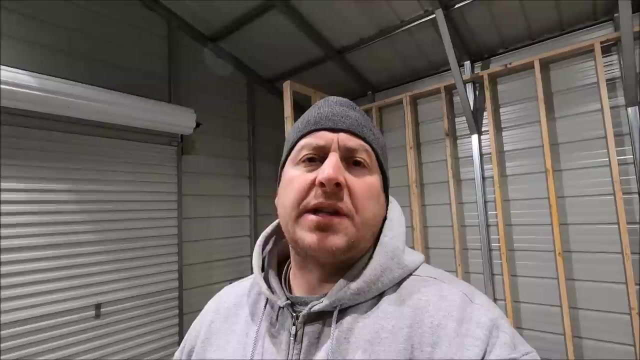 of what I'm going to be doing, which will also help those of you who want to do wiring at home. It's basically exactly the same principle they would use to wire light in a bedroom or, you know, down in basement projects or you know wherever you need to do wiring, So hopefully this helps. 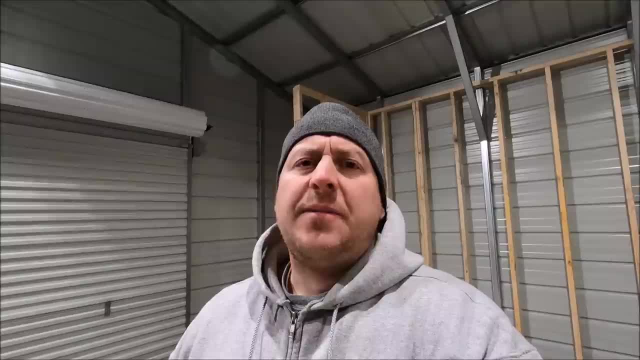 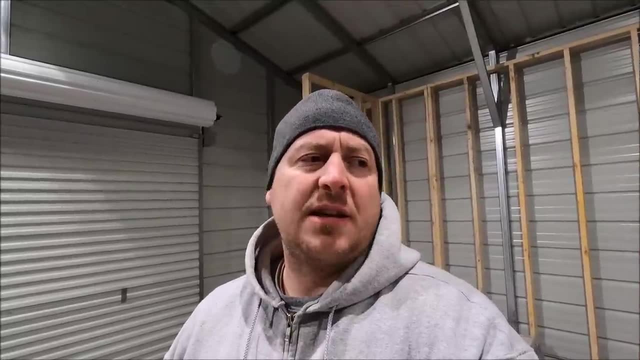 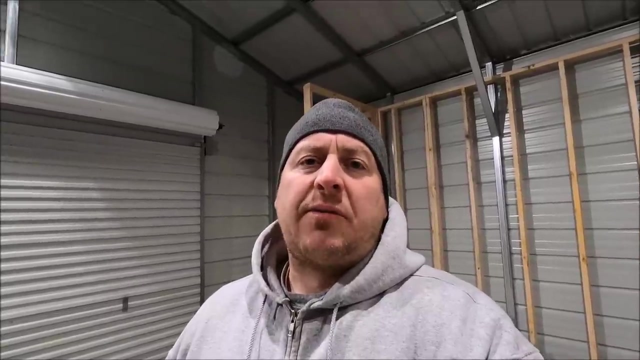 you out and, as with all my videos, this is kind of a you know, do this at your own risk. This kind of work is dangerous. I've mentioned it with the nail guns and with the table saw things like that. One accident can certainly change your life, but it's nothing that is to be afraid of as 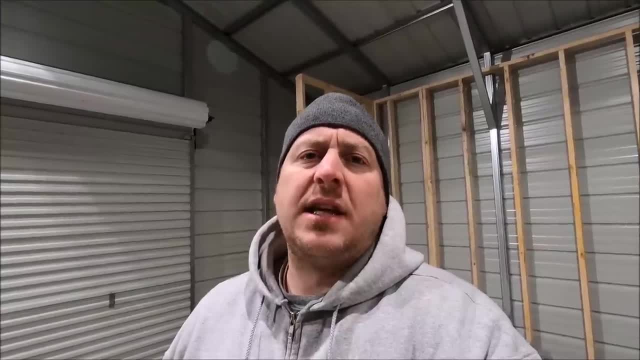 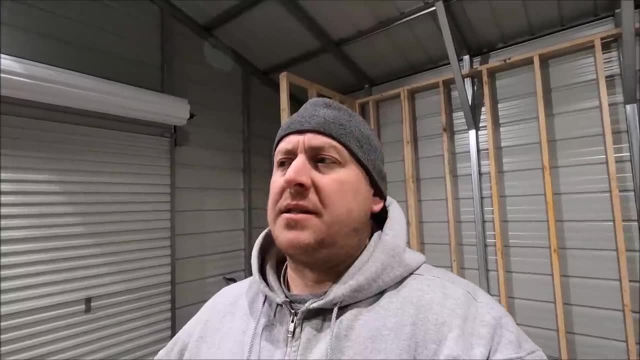 long as you just kind of respect the tools and certainly respect electricity, I know that this stuff really isn't that difficult to learn. A lot of people are just nervous because you know electricity is electricity and they always hear about people getting shocked and whatnot. but 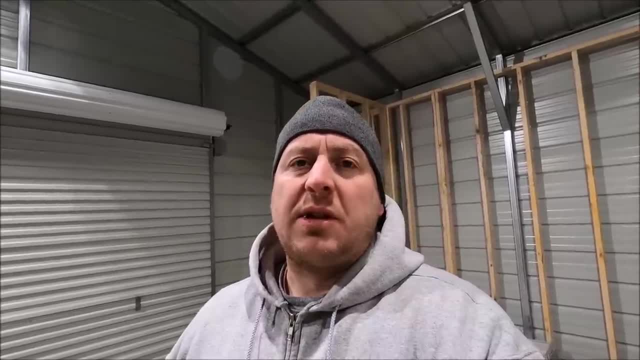 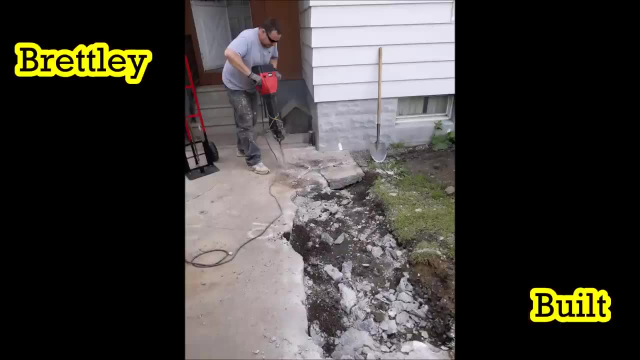 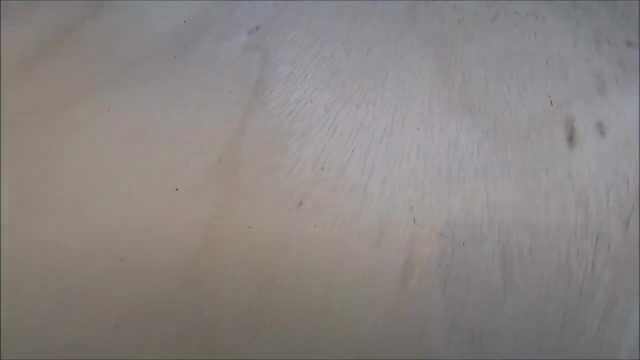 of course, do this at your own risk, but this is really something that I'm going to be doing. It's one of those simple things that pretty much anybody can figure out. I'm sure you're familiar with electricity, in that if you have a circuit, it has to be complete. 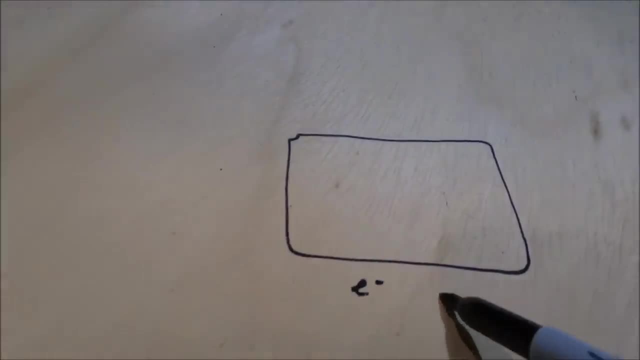 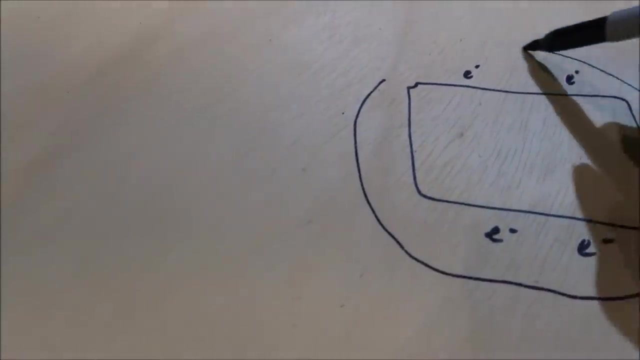 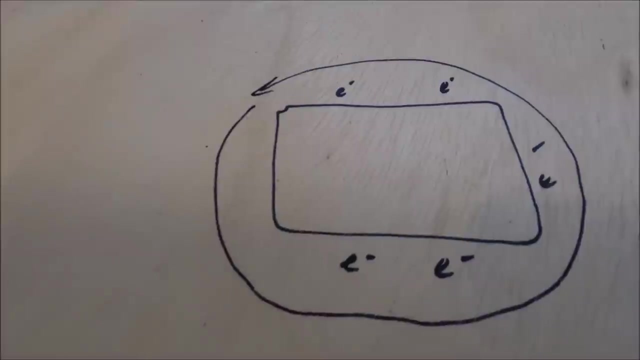 and current is nothing more than a flow of electrons around a circuit, and all these electrons do around the circuit, but in order for them to flow you have to have a closed loop, and that's one of the basic principles of electricity and what I use when I wire. 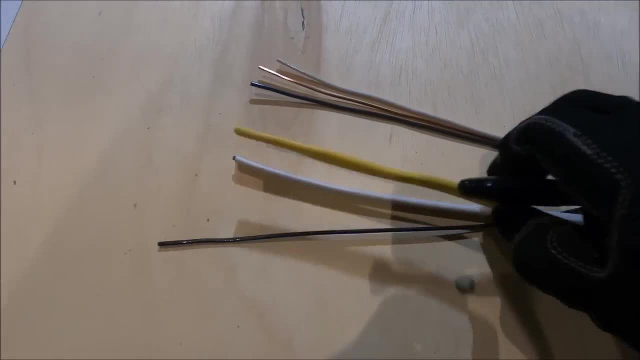 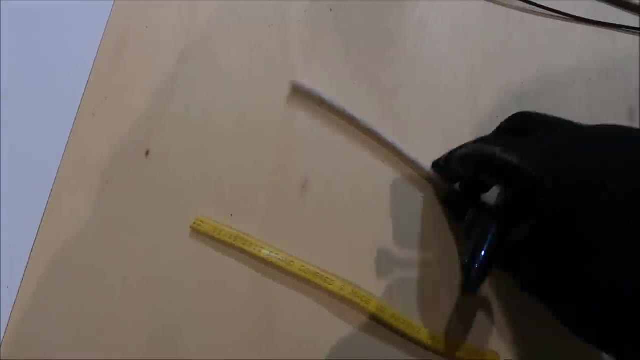 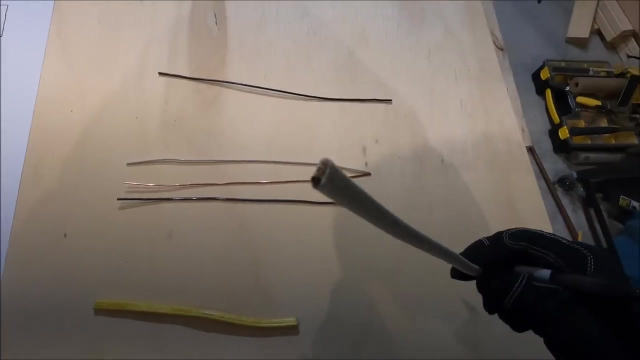 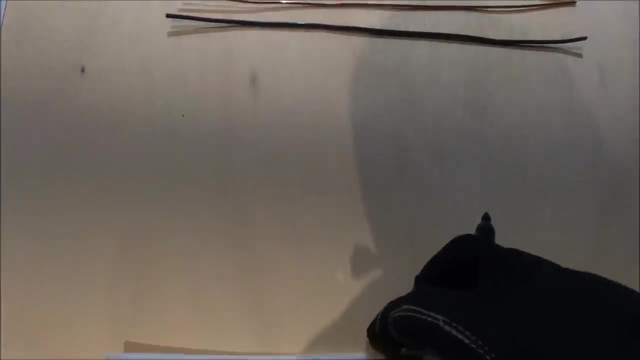 is this Romex. A lot of electricians they'll use individual strands, but I like the Romex because it comes with three wires inside. so I don't know if you can see that, but inside here there's three wires in this jacket and what's nice about it is it's basically one wire that can complete. 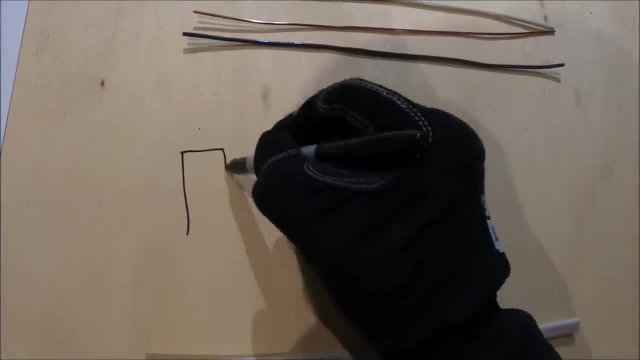 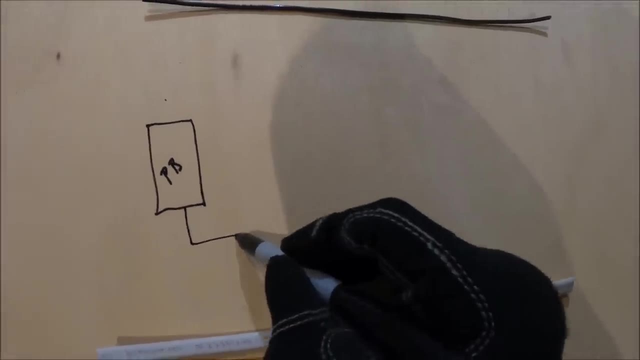 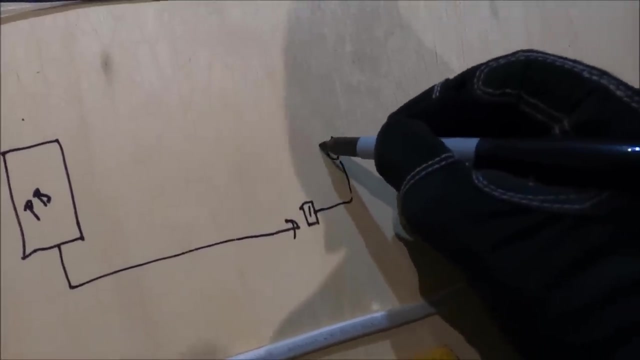 your loop, and what I mean by that is: let's take our panel box, or, in my case, out here. it's going to be a sub panel and I'm going to take power from the box to something like, say, a switch. then maybe I'll come over to a light and then I'll continue back. 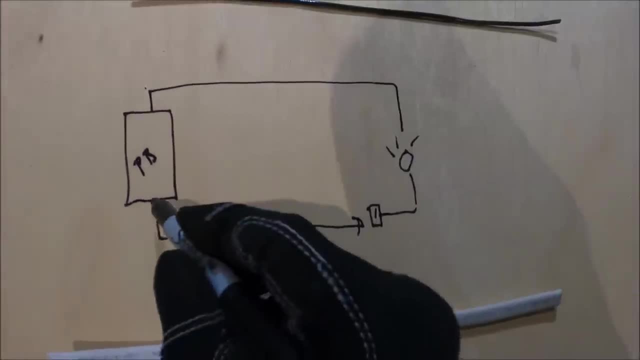 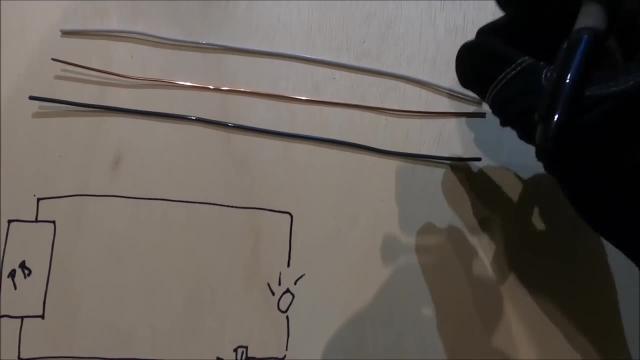 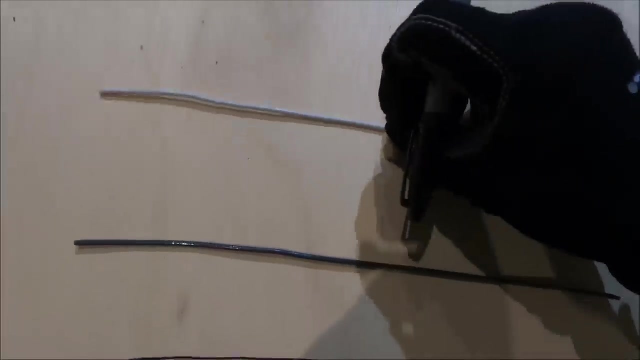 And in order for this circuit to be complete, the power has to leave the panel box and get back to the panel box. So with this Romex, it's really nice because let's take, just let's get rid of this copper wire. if I can grab it, it's freezing cold, so I have my gloves on. so now let's look at this. 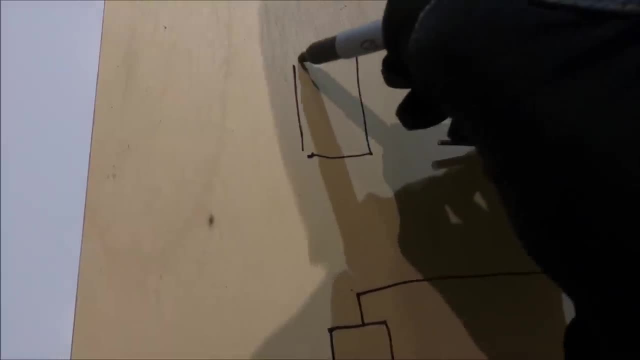 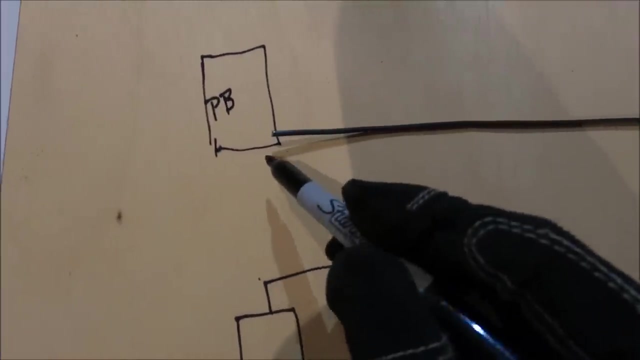 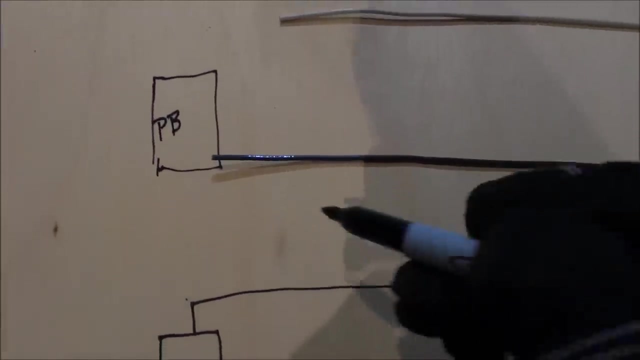 from the perspective of the Romex. so we have our panel box. Whoops, a little dyslexic today. The power leaves the power. when I say power it's, you know they might say a line's hot or where the electricity is coming from. so the power is coming from the panel box through the black wire and say 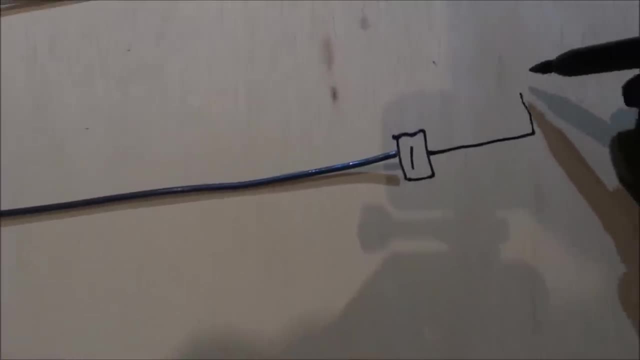 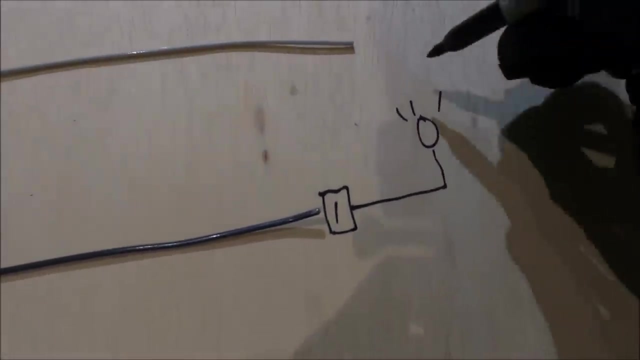 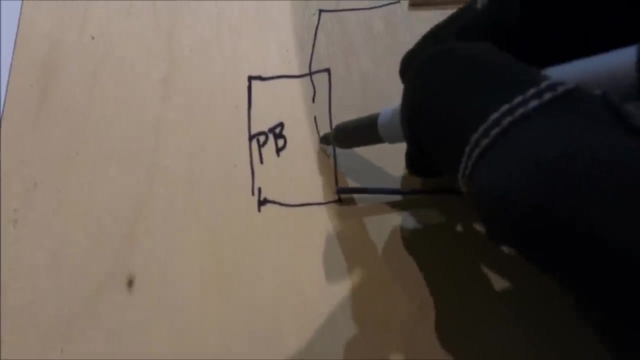 this is where our switch will be, say, we'll have another black wire that'll come over and hit our light, and then this is what completes our circuit is now it'll travel to the other side down this white wire and go back to one of the bus bars in the panel box. so the 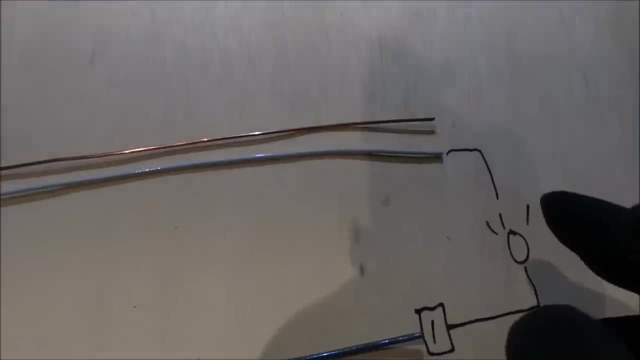 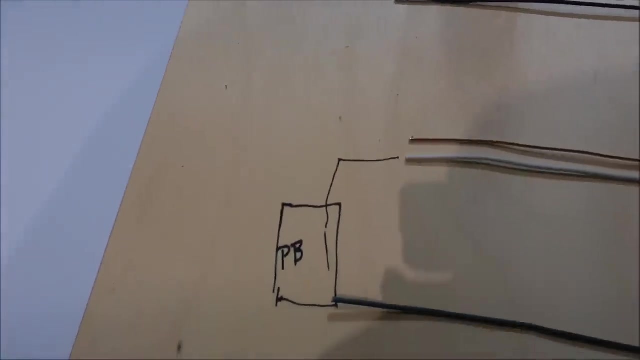 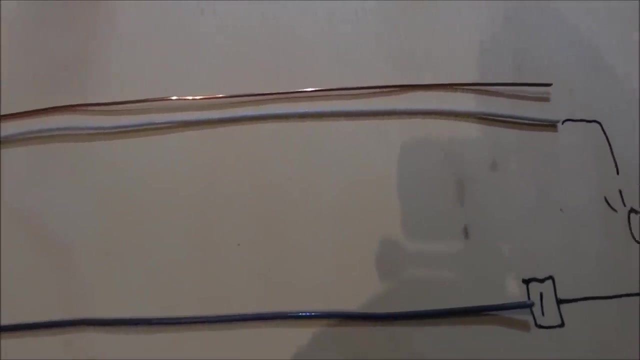 copper wire is your ground wire and it acts similar to the neutral wire. it provides another avenue for the electricity to get back to the panel box and complete this circuit in outlets. it's a safety thing instead of you becoming the short circuit and going from the hot to yourself and and hurting 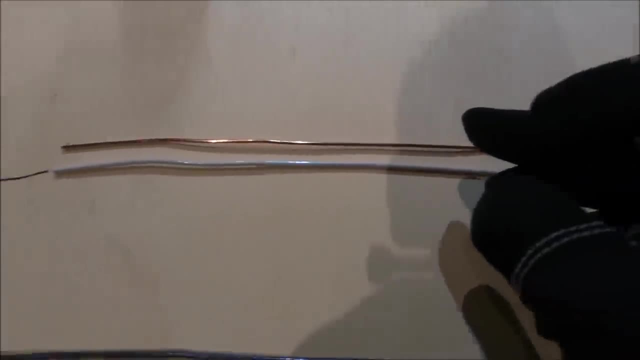 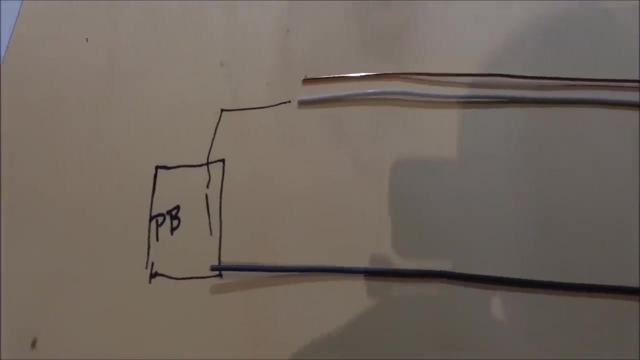 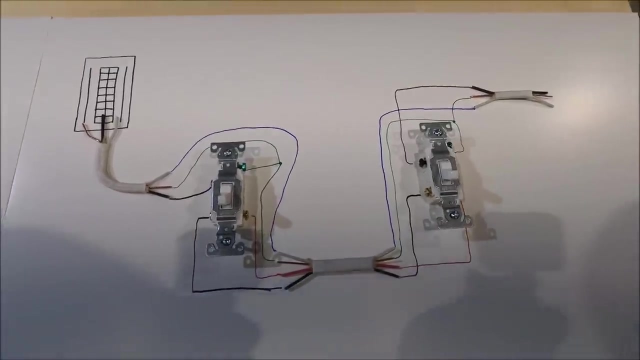 yourself. it'll actually provide another avenue to get the electricity back and since this copper wire is more conductive than you are, it'll make it back to the panel box and down to the ground safely. okay, so I drew out some circuits here that are gonna represent the circuits that I'm going to use, the 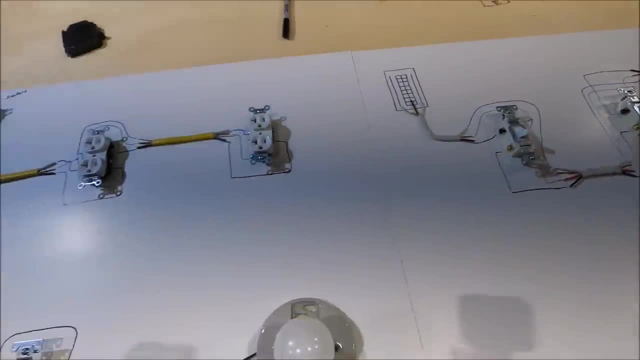 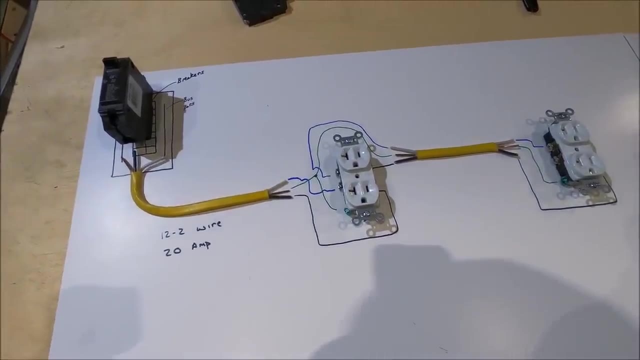 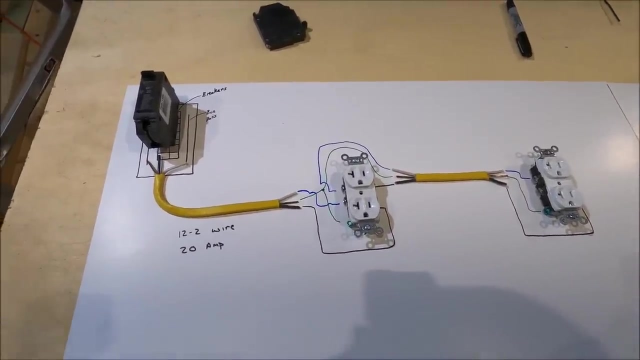 smaller circuits I'm going to use in this building. there's a few more, and a few people have reached out to me asking me some questions on YouTube and I'll create another video that gets a little bit more involved. but the one thing that I want to preface is I I'm not one of these guys that take 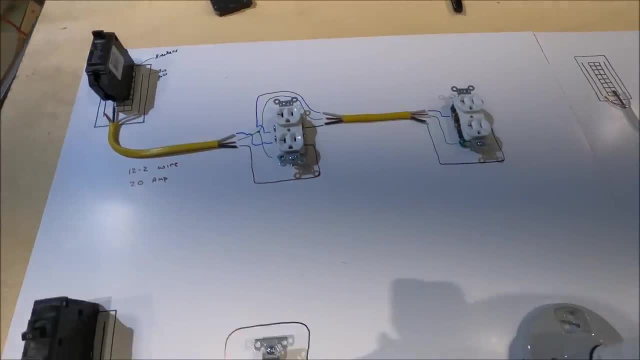 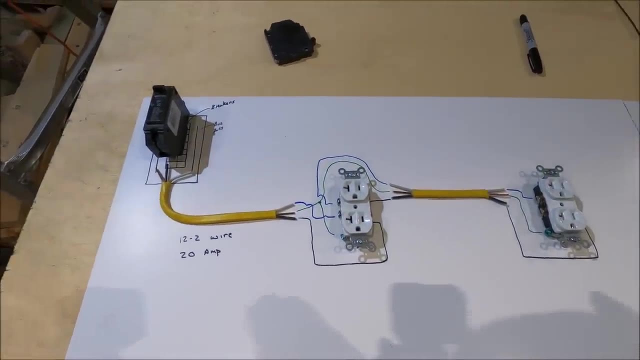 shortcuts with a wire. there's different ways to wire these circuits to save some wire, and for me I just like it to work 110% of the time, and so I absolutely won't. you know, use the. if you look up some of these circuits online, people. actually take the neutral wire and they'll make it a hot to get it to run back and run a switch or something like that. I don't do stuff like that. a lot of other spend the extra a couple dollars and just make sure it's gonna, it's gonna. 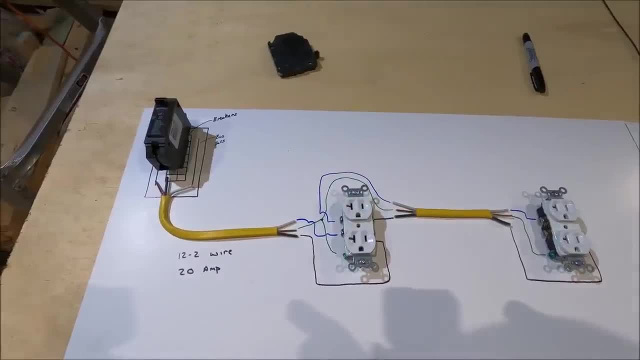 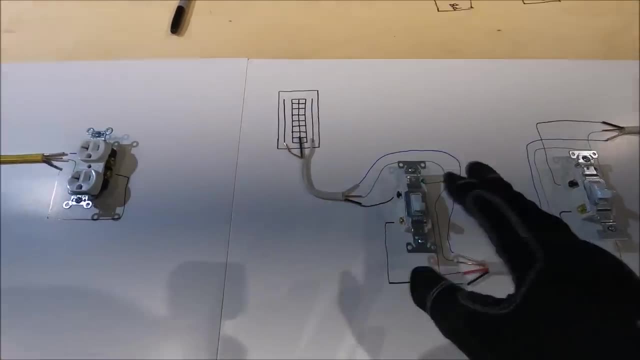 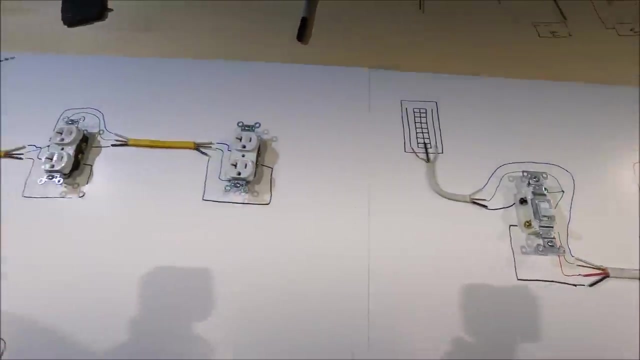 work regardless. but I've come into rewire houses before and do different things and you have to sit here and play these little games and figure out where you know where the wires went in these circuits, because they decided to use the neutral as a hot wire to go back to lights and different things like that. so 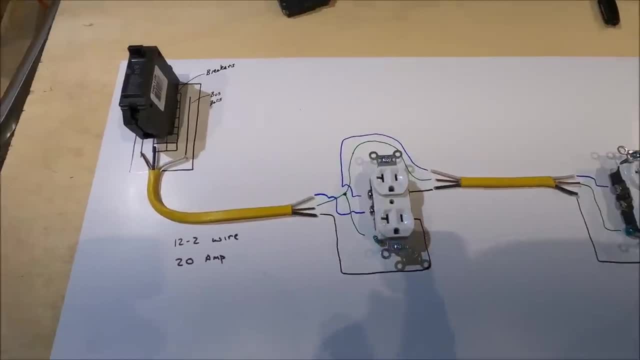 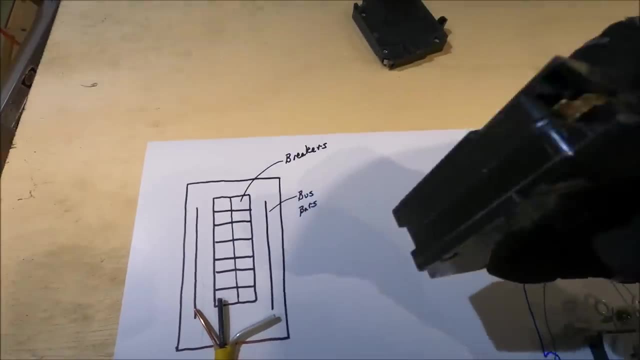 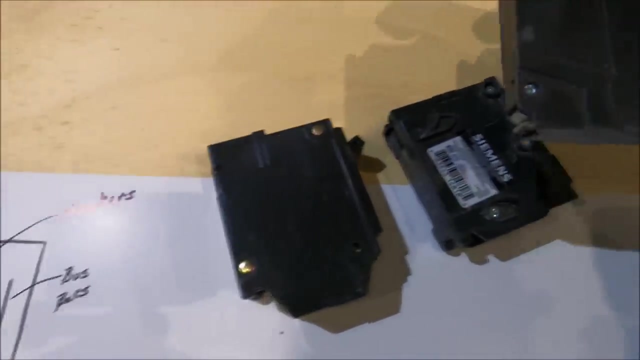 just for ease of the next person. I certainly don't like to make things more complicated. they have to be. so start out with a little panel box that I made here and these breakers put out a couple breakers here and they're all a little bit different and you can. 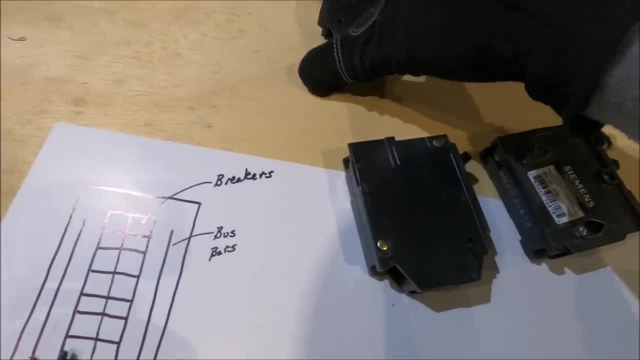 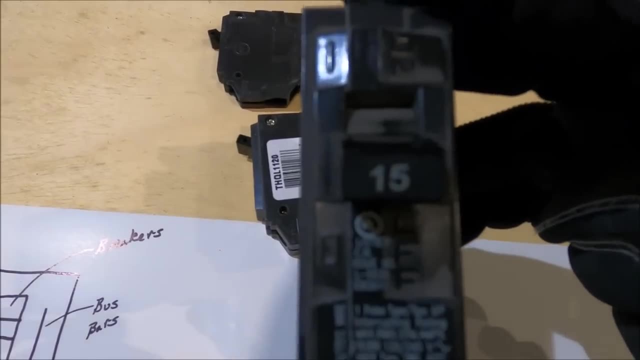 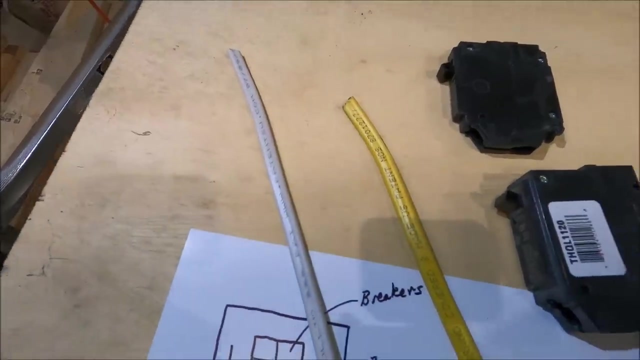 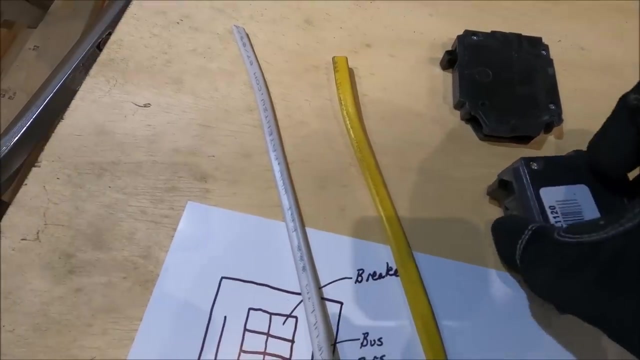 tell there's. they're always marked- what the amperage is. the voltage in these circuits is always 120 volts, but the amperage is different, and that's what you want to pay attention to. the white Romex is 14 gauge, 15 amp wire, and the yellow Romex is 12 gauge, 20 amp wire, and so, whenever you're, 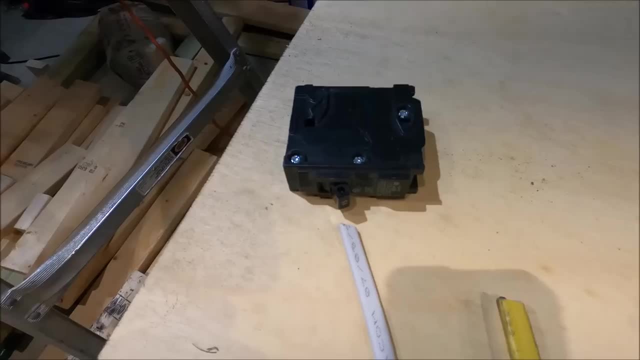 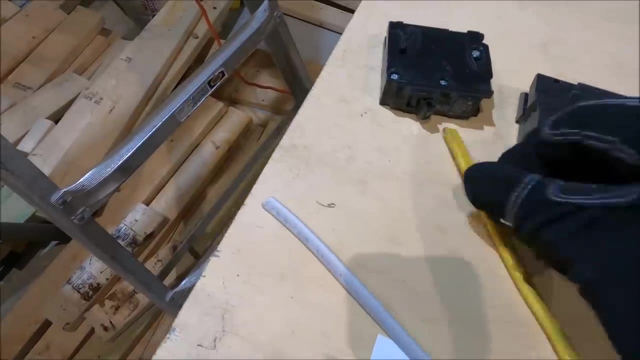 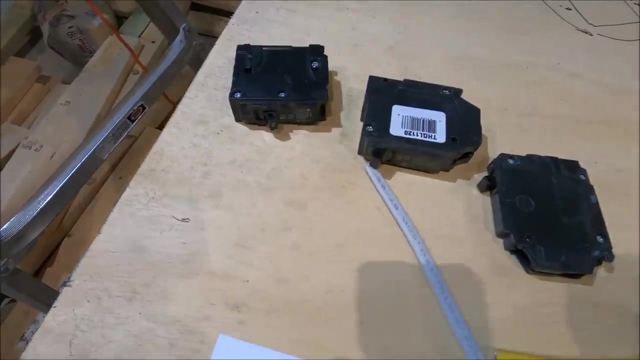 running these circuits. you want to make sure that you, that you pair up the proper breaker size with a proper wire. you can always say, put the- you know- a larger wire on a smaller breaker and that's not a big deal. but you never want to go the other way and say, put that 14 gauge, 15 amp wire on a 20 amp breaker. 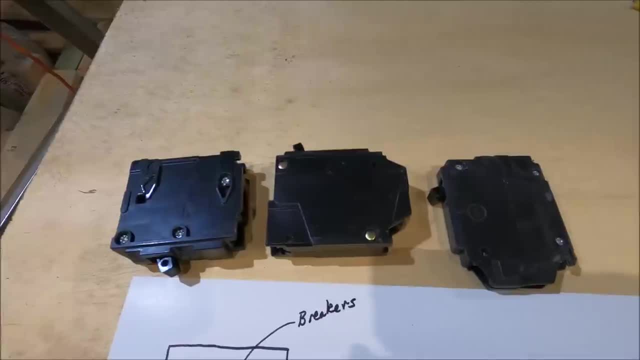 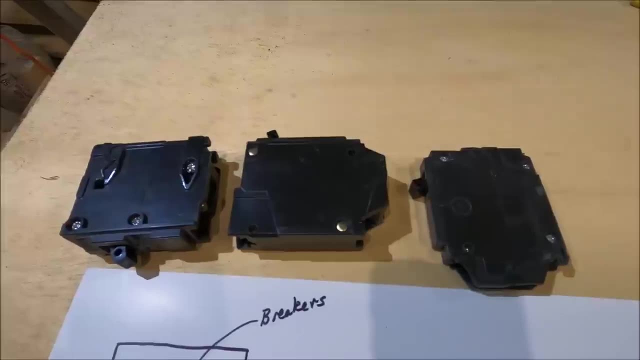 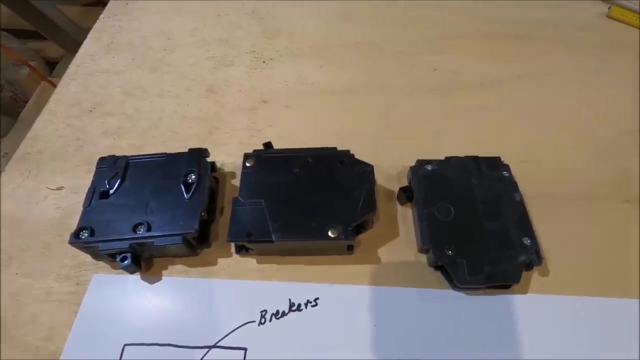 then you could potentially cause a fire. one thing that you do want to pay attention to with the breakers: a lot of them are well, they're all kind of specific to certain boxes, and so you want to make sure that you use the correct breaker or the compatible breaker for the type of box you have. so 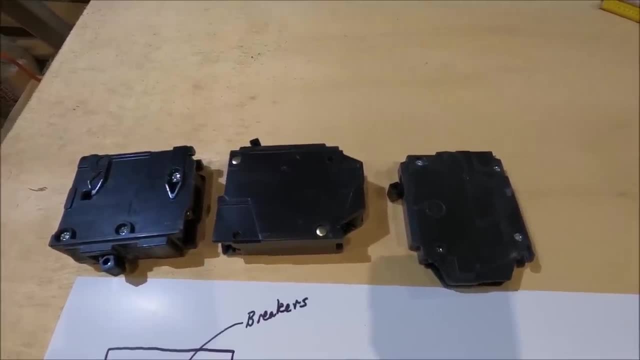 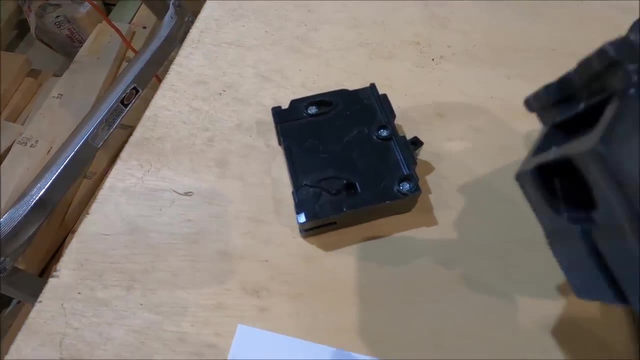 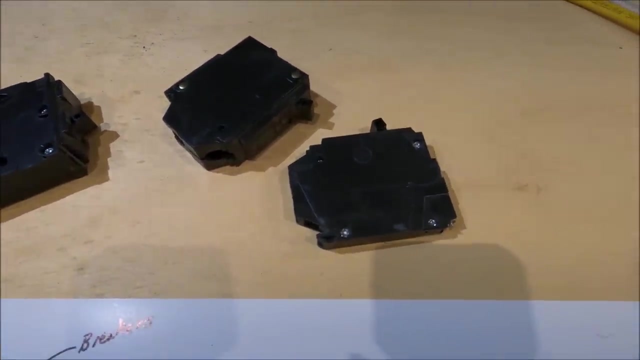 if you have a general electric box, you may not be able to use a Murray breaker in there, and you can see some of the connections that they'll make inside the box are a little bit different. they won't always hook up the same way and so you definitely, when you go to you, know if you want to run an extra circuit for. 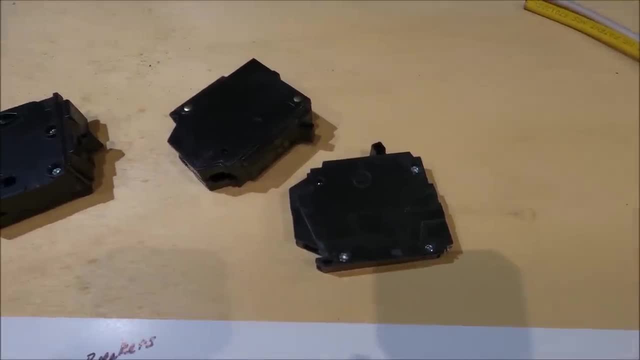 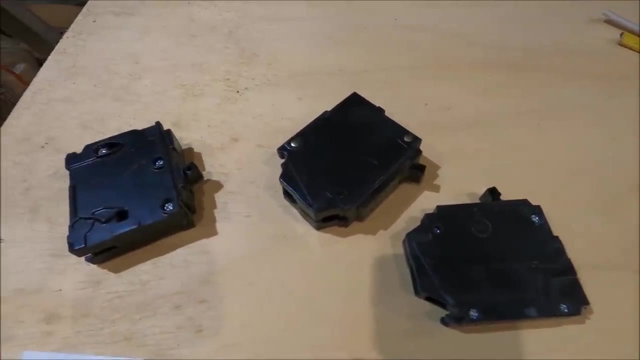 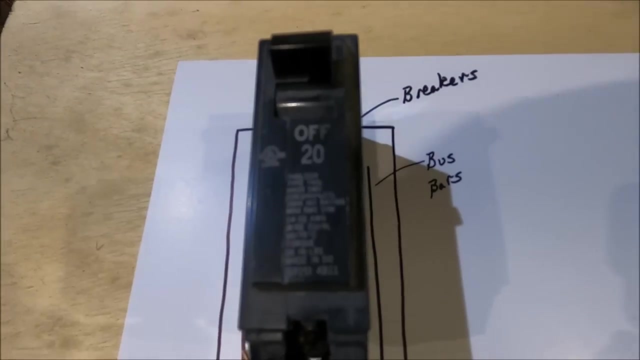 whatever you're doing- a garage or basement or whatever you want- to make sure that you select a select a compatible breaker to hook up the circuit in your panel box. okay, so here's my little panel box drawn out. I'm gonna use a 20 amp breaker and you'll see that, just like in my last video. 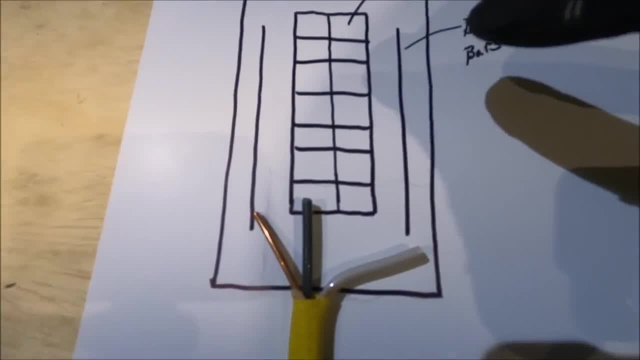 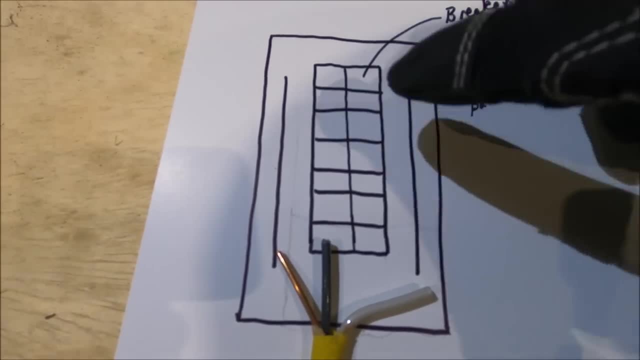 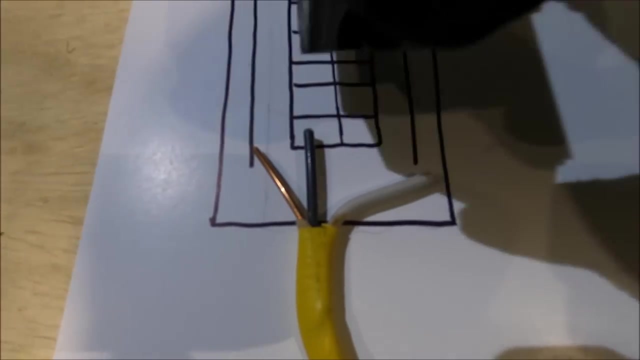 I have my little bus bars here on this side, so for for my sub panel I had to separate the neutrals in the hot. so I have the white wire, the neutral going to one bus and the ground going to the other bus, and my breaker in the middle. 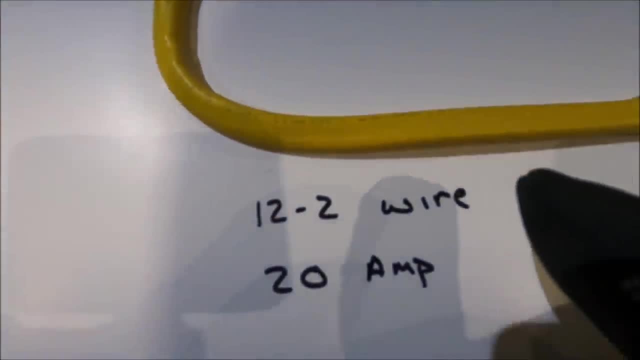 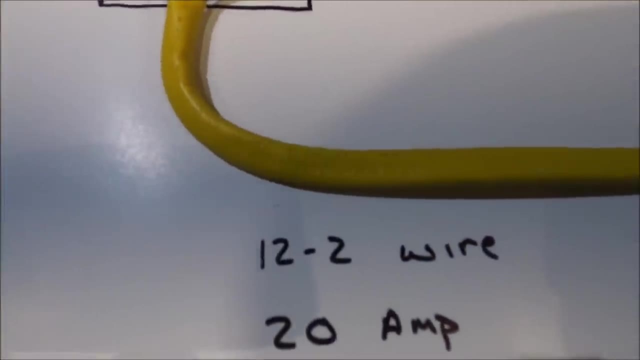 20 amp breaker with my 12: 2 wire and 20 amp or 12 gauge wire and my 20 amp wire. so you'll notice the bus bars are in the middle and the two bus bars are in the middle, so you'll notice that they have two bus bars. 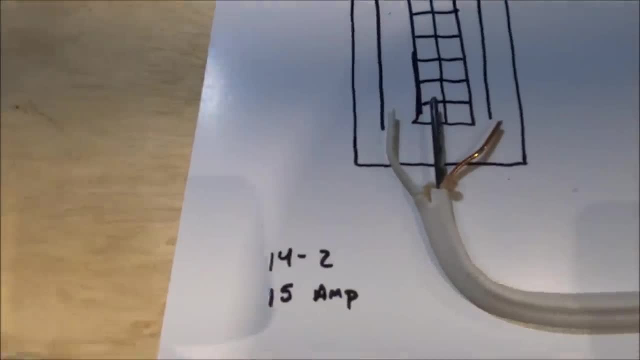 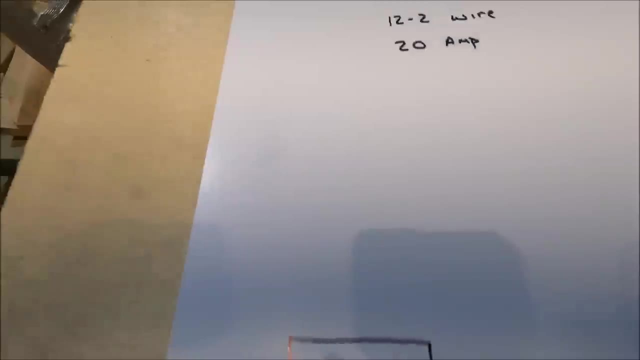 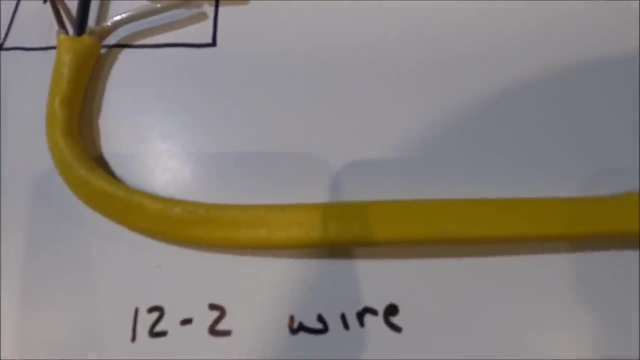 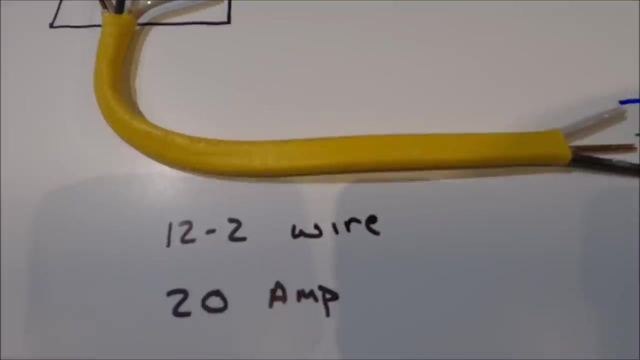 wrote 12-2 here and you'll notice i have 14-2 down by this white wire and it's a little difficult to understand at first. you'll notice that there's three wires in this yellow romex, so why would we call it a 12-2? well, i don't know that people that manufacture this, or whatever they you know. 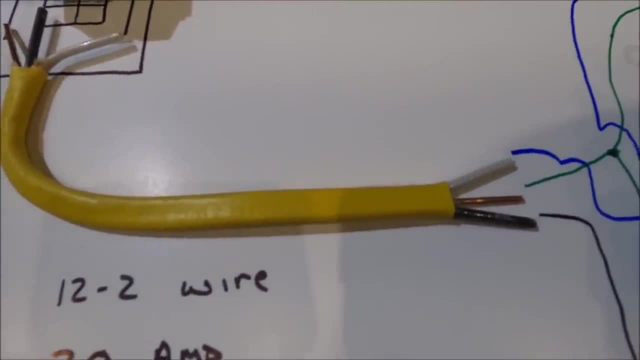 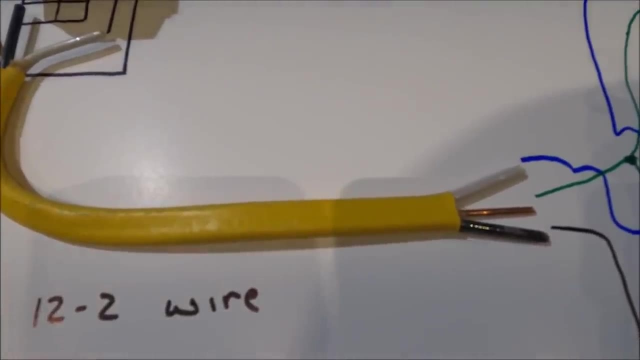 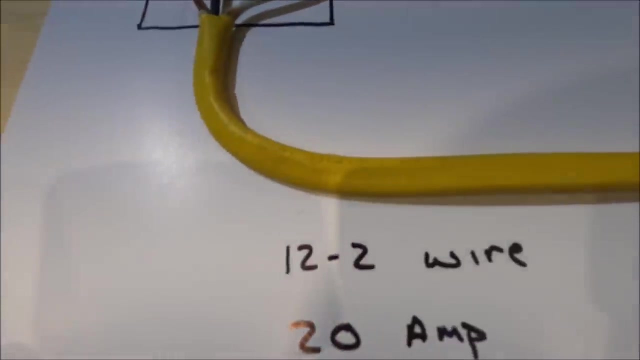 electricians or whoever came up with this. i guess they're only considering the two wires that are used to, like the two main wires, to transport the or to conduct the electricity, and so you don't count the neutral wire, or you don't count the ground wire, and so this is a 12-2 wire, because 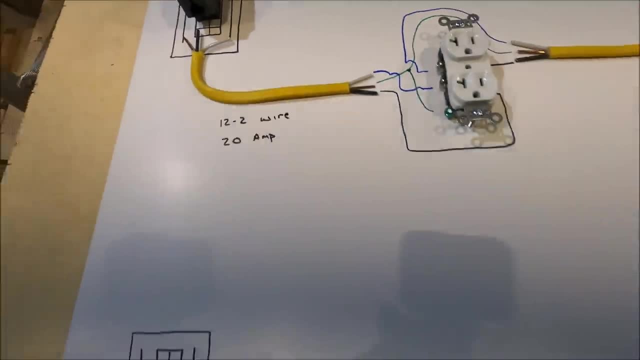 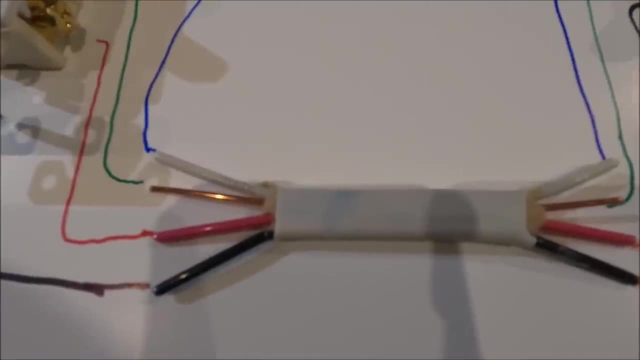 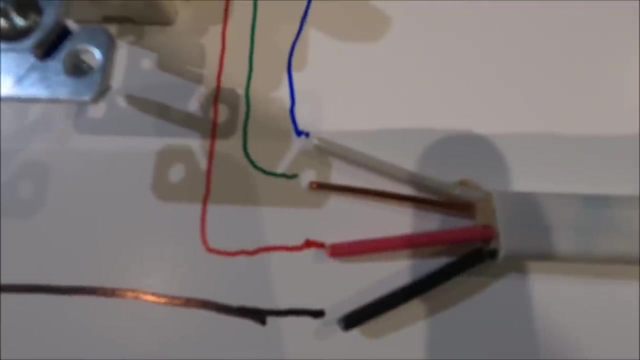 it's 12 gauge wire and there's two wires inside. if we come over to this little wire, you notice it's white, so it's 14 gauge, 15 amp wire. but you notice that it has another red wire. it has a red wire, so there's a white, red and a black. 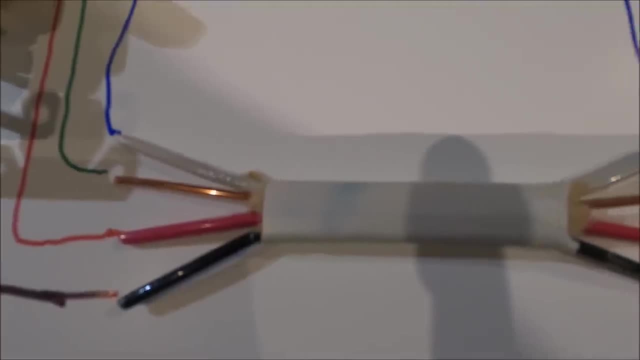 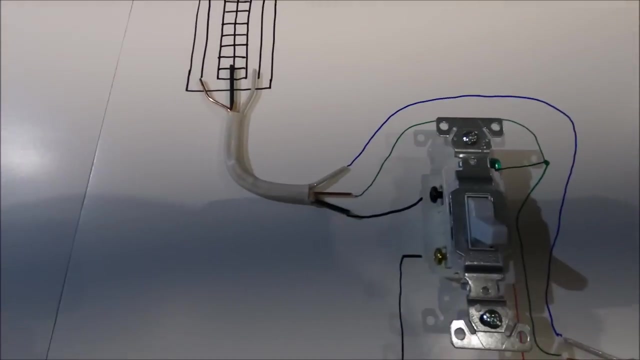 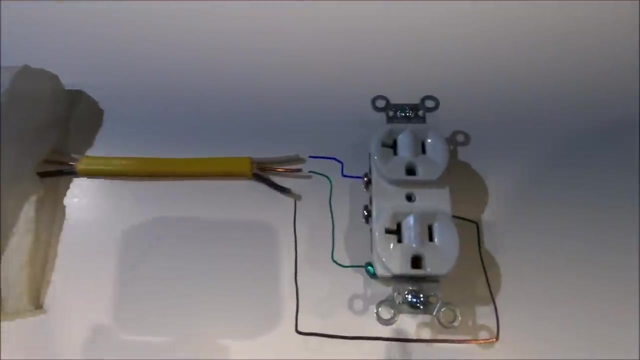 wire, so this is going to be called 14-3 wire- three wires, not counting the ground, and that's very important when we get to this circuit, which is going to be a three-way switch. okay, let's start with the typical outlet wearing a typical outlet in your home. so this is a rated for. 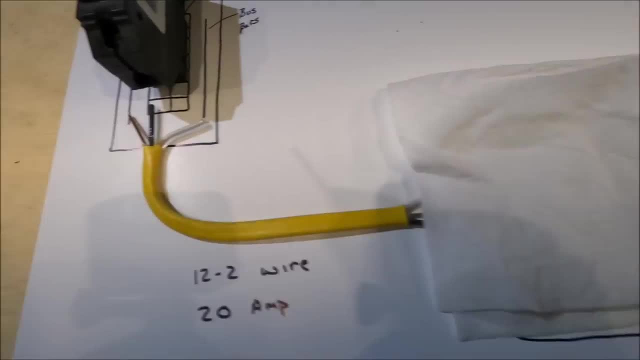 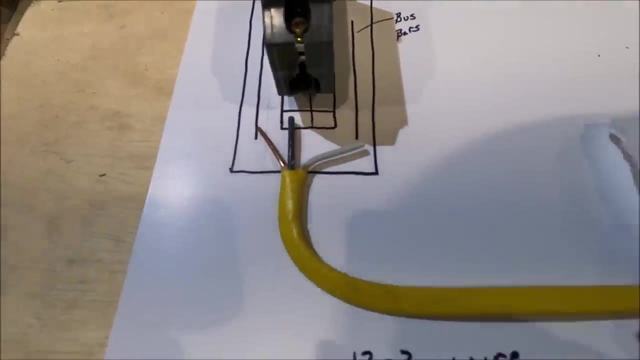 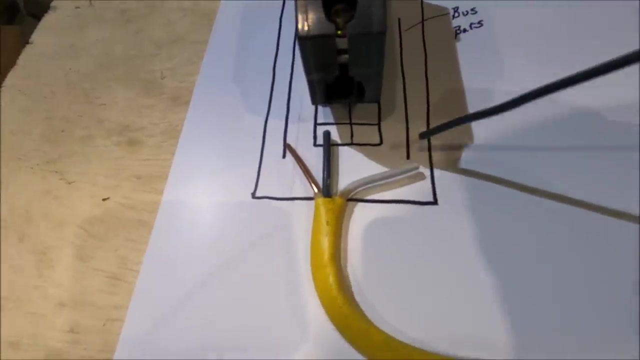 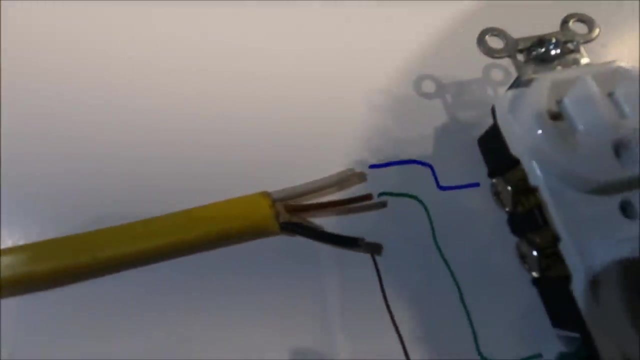 20 and amp circuit. so, like i said before, we have our panel box or sub panel hooked up. so let's discuss what's actually going on. to hook this up, we hooked up the black to the breaker and then we hooked up our other two wires to the buses. then our yellow wire comes along and i use blue instead of the. 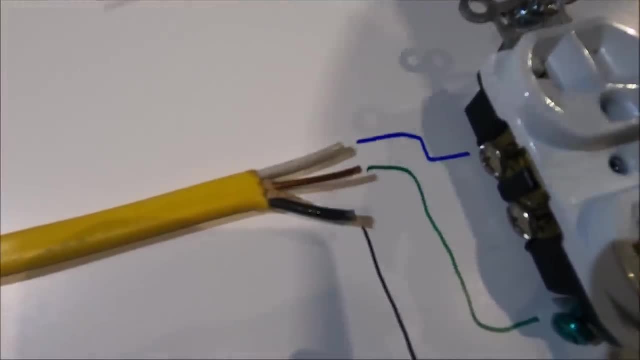 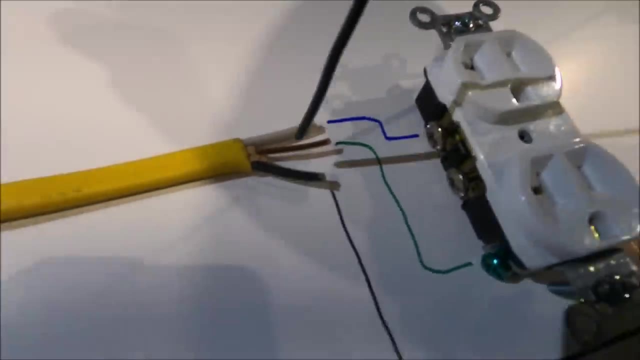 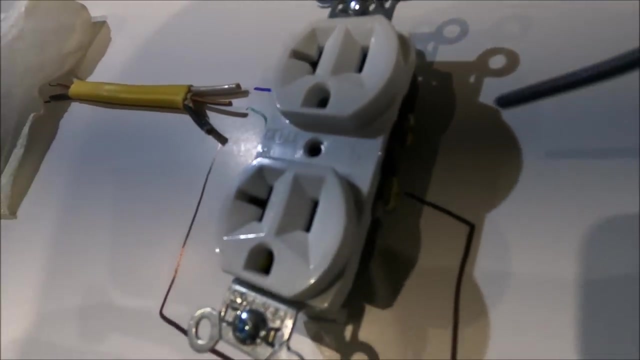 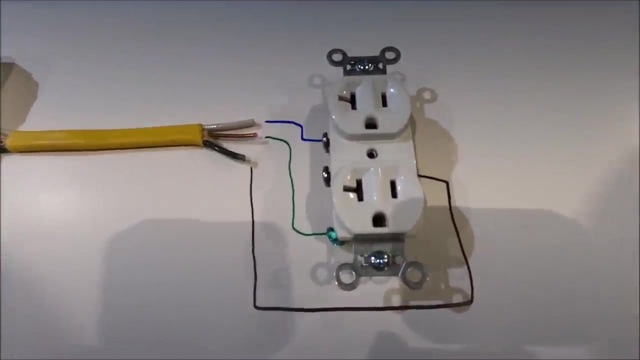 white wire just because i obviously there's no way to draw white on white. so i have the white wire that i hook up to the silver screws, i have the copper wire which is hooked up to the ground screw and i have the hot which is connected to the copper screws. so this is very standard. if somebody hooked this up backwards, it's not a. 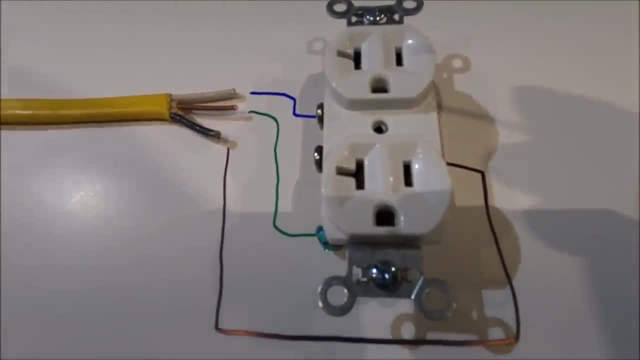 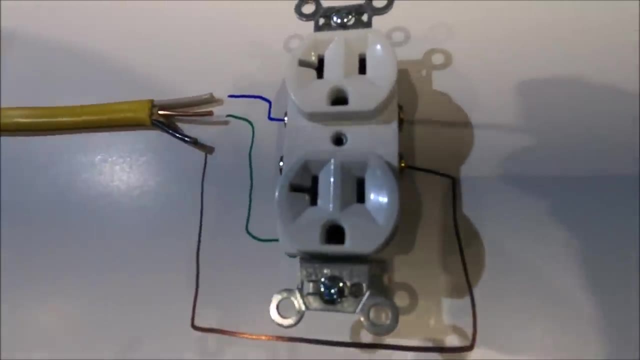 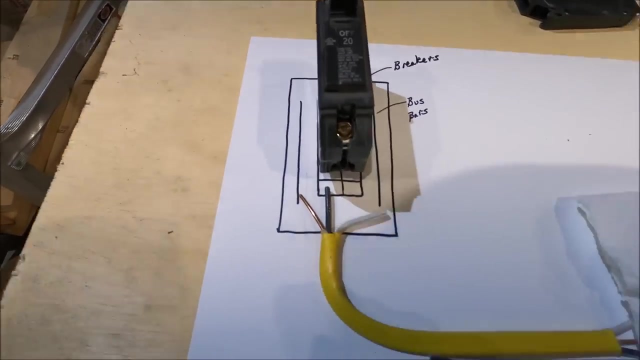 huge deal. ac power is pretty forgiving. there's a whole theory behind it. so if you connect them backwards, um, just connect them back the right way. i don't really want to get into the theory on how all this stuff works in this video. so whenever you turn the breaker on, it's going to make the 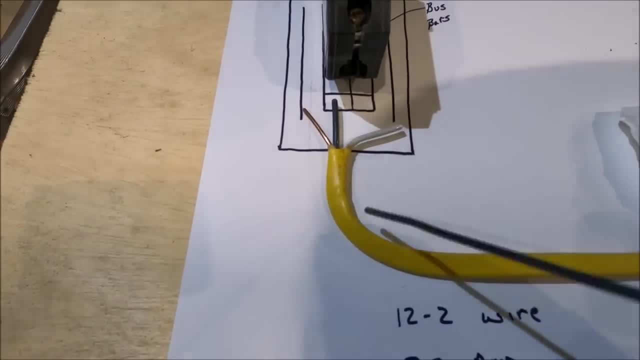 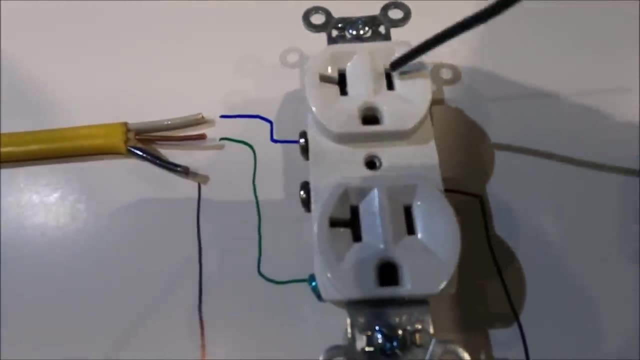 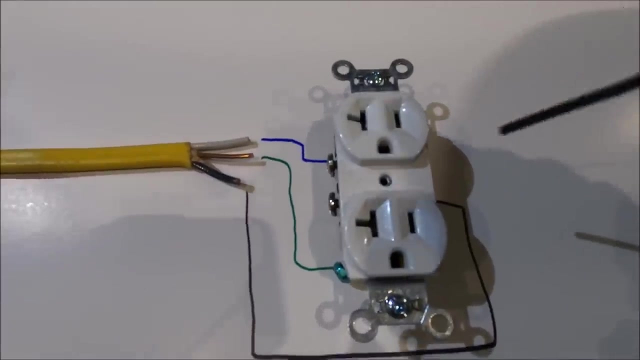 circuit hot, which means through this black wire is going to have power to it. it's going to power clear up to this screw and then to the terminals here and as soon as you plug something in here you're going to complete the circuit. so if you plug in a lamp and turn the lamp on, 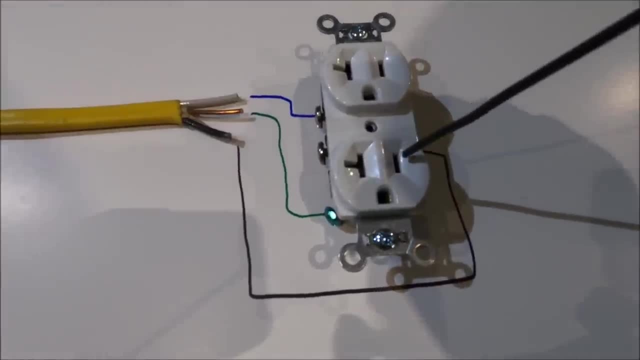 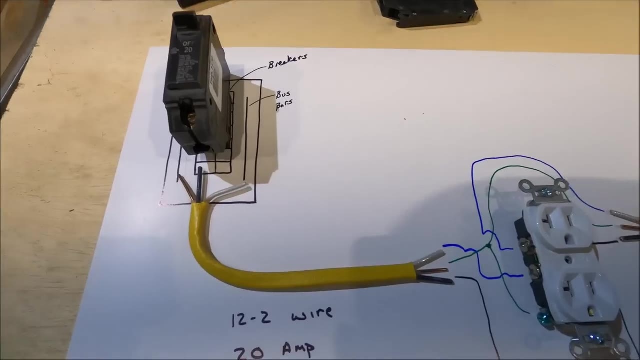 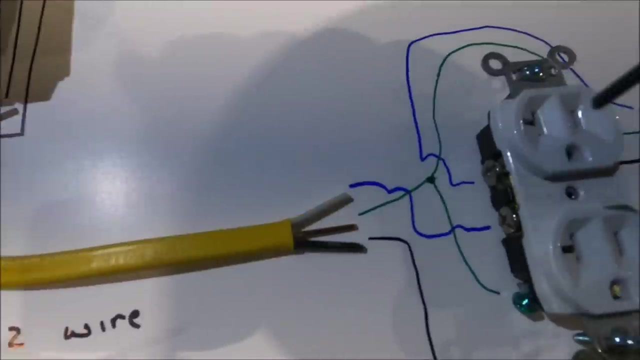 your power is going to flow through the black wire and it's going to go through the lamp. come back to the neutral and then head back out all the way back to your panel. okay, that was for a single outlet. for two outlets it's not a big deal. same, same process. come over to your first outlet. you're. 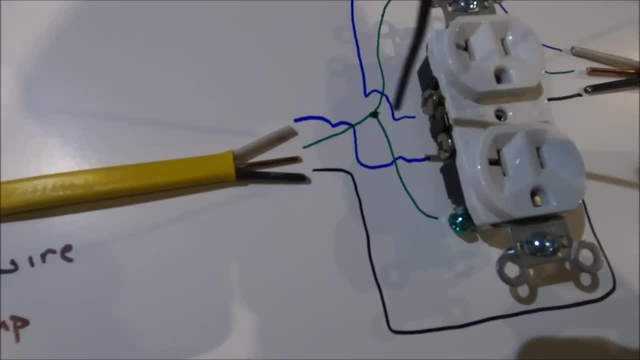 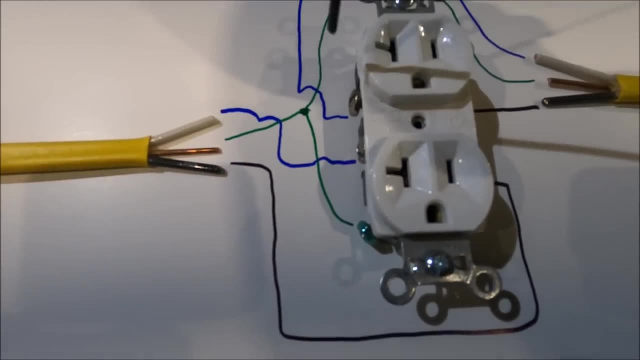 going to hook up your neutral to the silver screw and you're going to hook up the black wire to a copper screw and then, with your black wire, you're going to hook up the silver screw and then with your other screws- kind of follow me on this- your other neutral is going to come up and hook up to the. 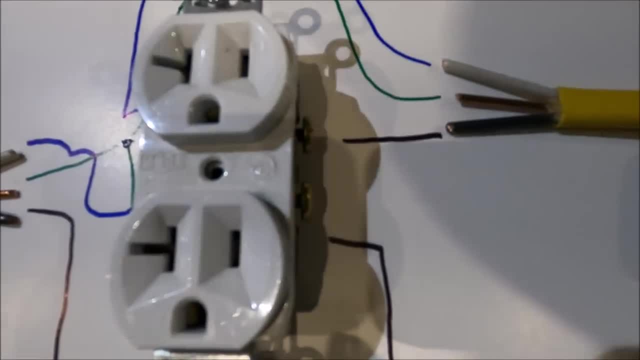 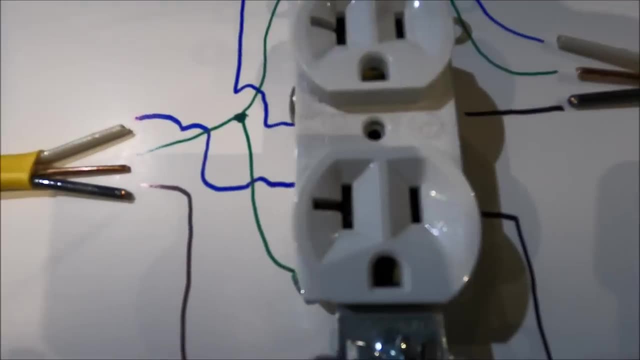 silver screw your other black wire is going to hook up to the top. i would recommend trying to stay consistent. make sure that if you hook this black wire up to the top, hook up that other neutral to the top of the silver screw, and then this wire would go to the bottom, this other. 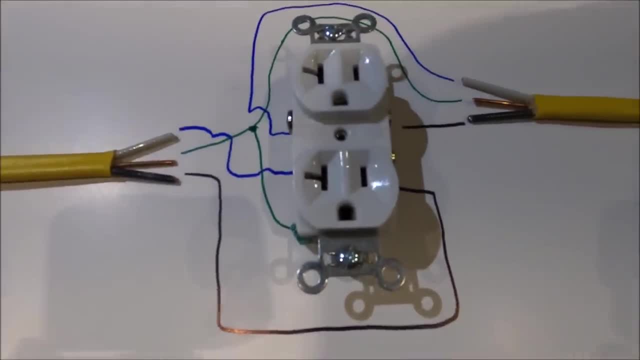 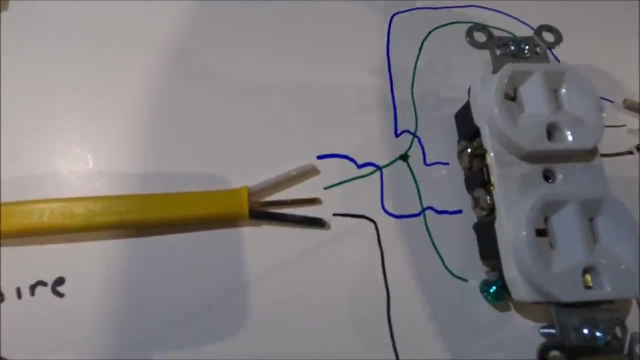 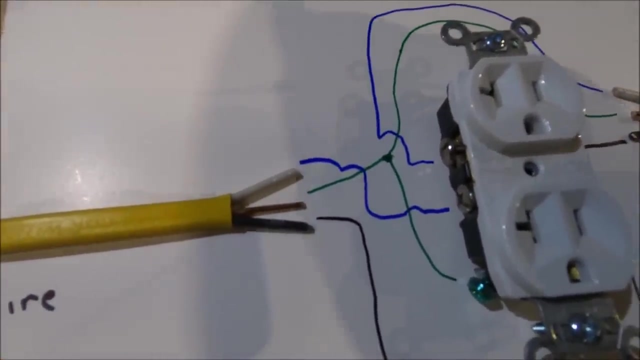 screw would go to the bottom, just trying to stay consistent when you do electricity and try to keep things neat so it's easy to follow. here you're going to have to actually watch that wire, nut these copper wires together because, as you'll see when I go to 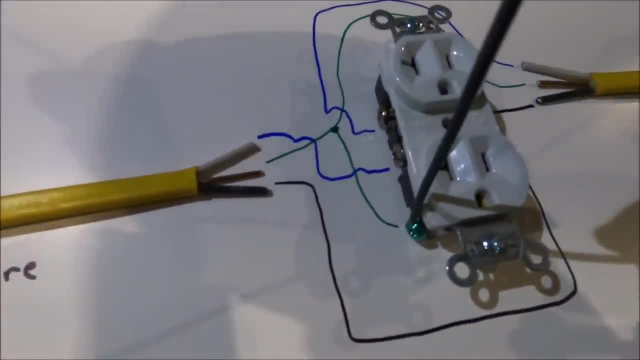 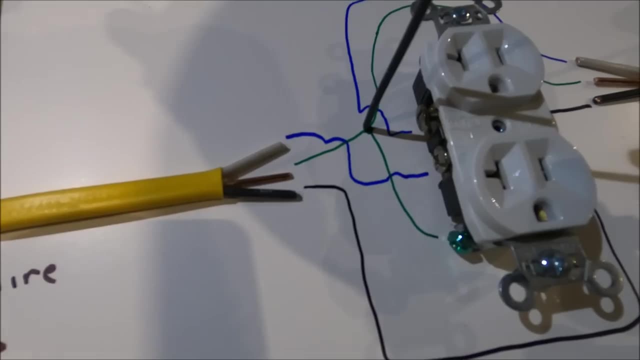 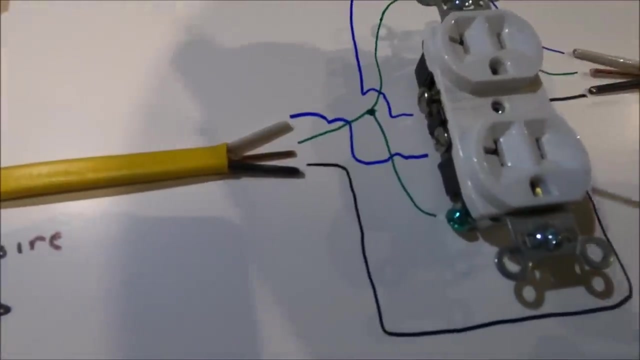 actually wire the building, you'll notice that there'll be a wire off from this copper wire coming off, this be wire nutted and then this new, this ground will come in, then this ground from this other wire will come in. it's not good practice to put two wires on one screw, and so what you do is you kind of make a 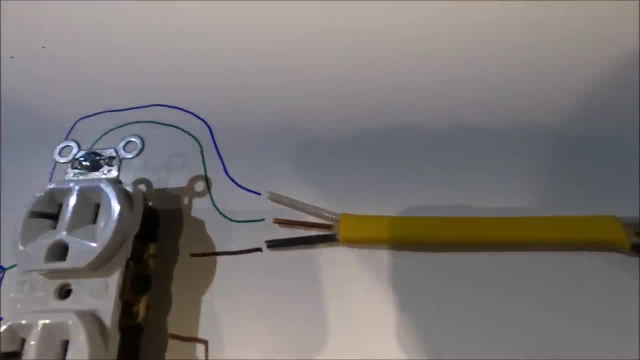 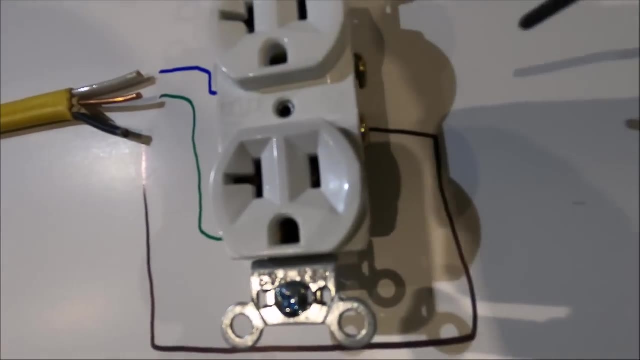 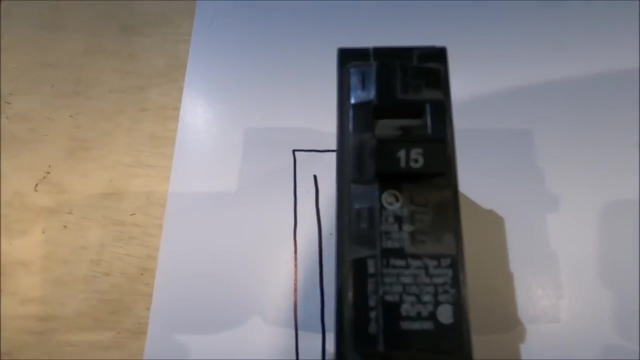 pigtail here and connect them all together and then heading down the circuit back to that, the last circuit, same principle as before: just hook it, hook it up and just terminate the circuit at the end. okay, now we're gonna hook up a light and you guessed it, we're gonna use a 15 amp circuit with our 14. 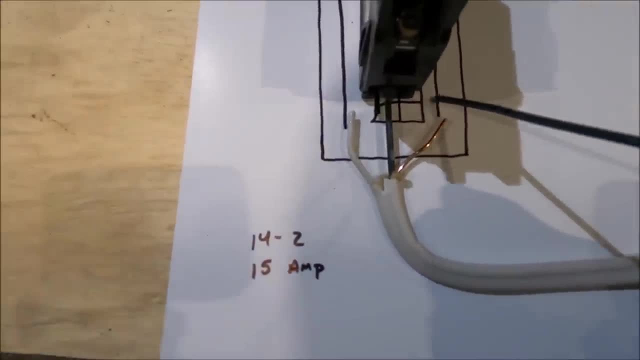 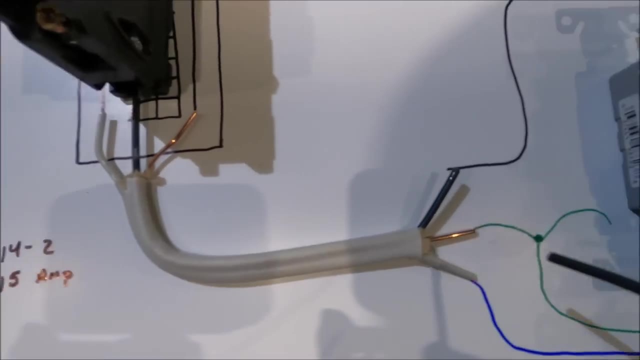 gauge wire. same principle as before: we're gonna hook up a ground to a bus, neutral to a bus, and we're gonna hook up the black to the breaker and we're going to come over to the switch. Let's start with the ground this time. 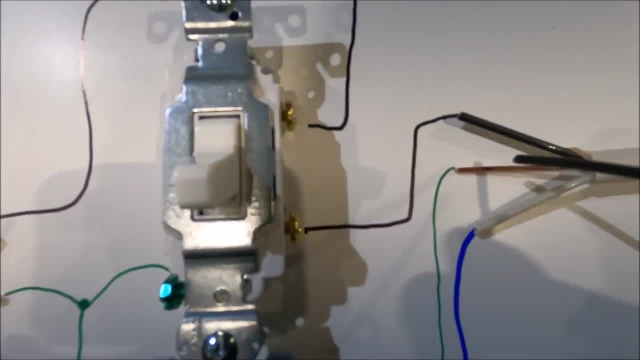 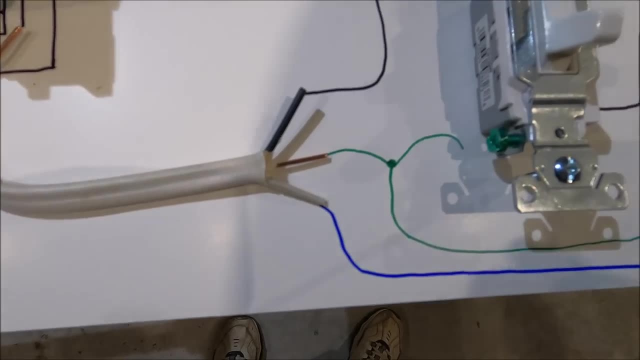 Remember we had a ground on the last circuit. we had a ground wire and a ground wire from two different wires. What we're going to do is the same thing: We're going to create a little pigtail and bring the two grounds over and we're going to wire, nut them together. so we've stayed safe. 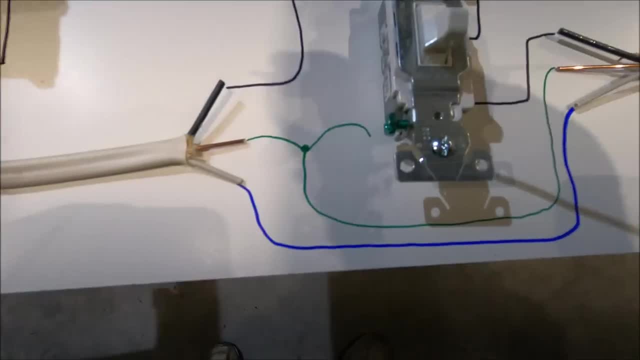 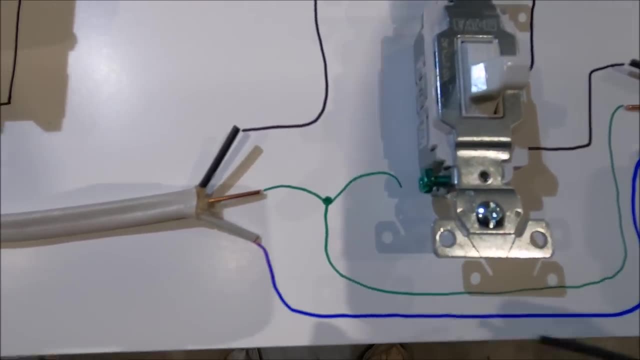 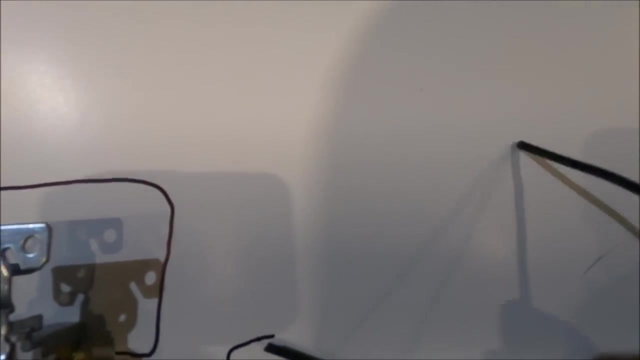 making sure that there's not two wires on one screw. Then we're going to hook up our neutral wires, and the reason is because the neutral wires aren't going to break the circuit. It's the hot black wires that are going to break the circuit. So, as we were talking before, you have a circuit. 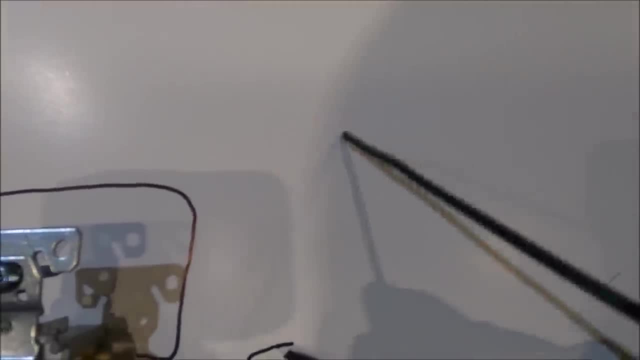 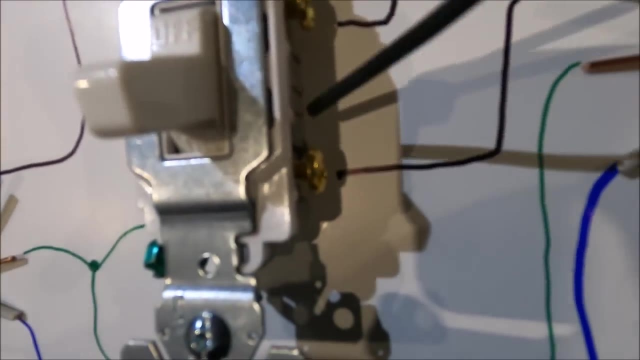 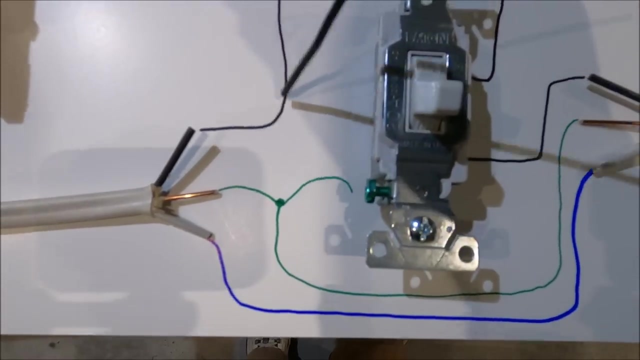 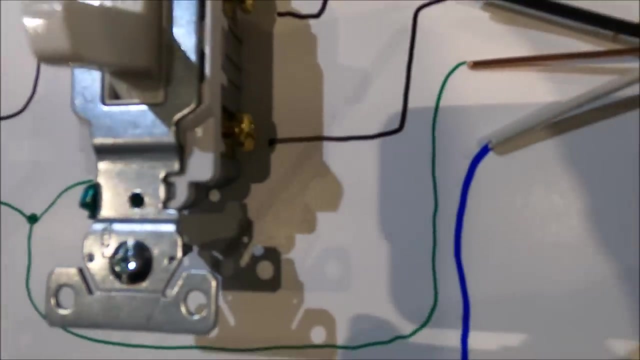 and as long as the electrons can flow around, or as long as the power can flow around in a circle, you're good. What the switch does is break it at a certain point, so the circuit's broken and your light turns off. We'll do is we'll hook the one black wire up to the first screw and then we'll bring the other. 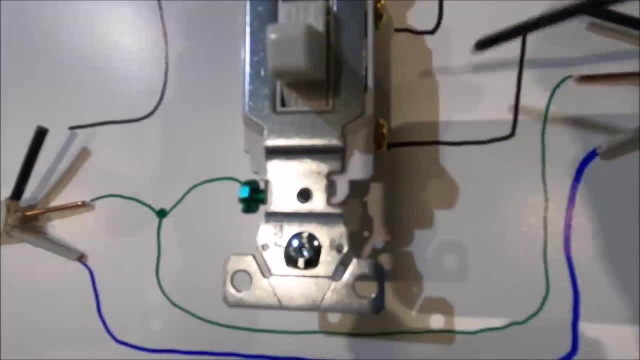 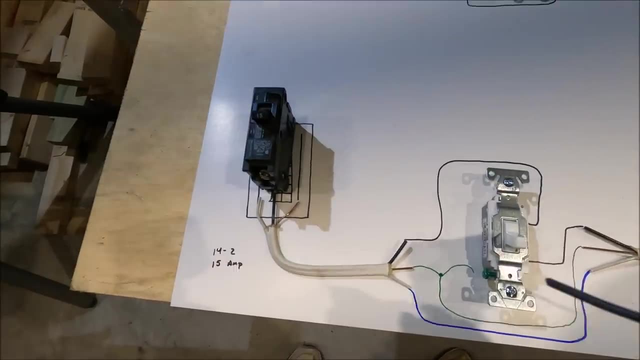 black wire over to the bottom screw. It really doesn't matter which side you want to put these on, because all you're doing is breaking the circuit. Nothing's really specific here, and so what's happening is, when you flip this breaker on, we'll go ahead and turn our breaker. 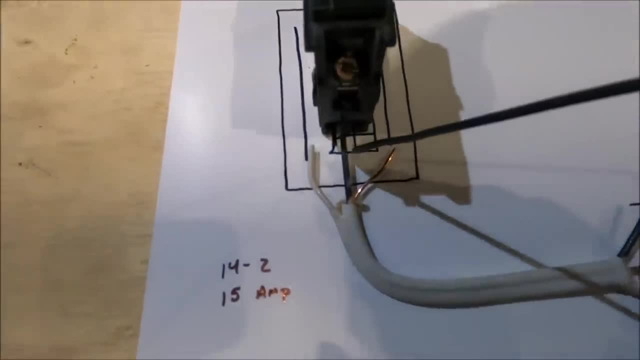 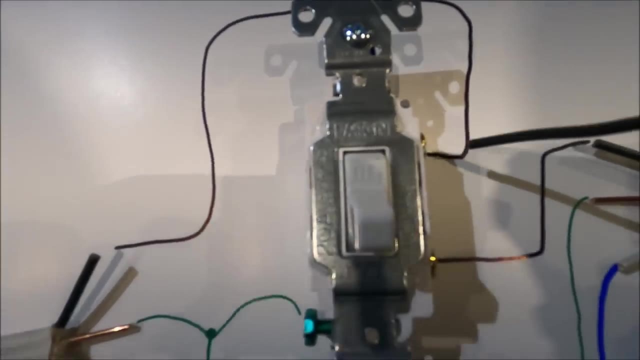 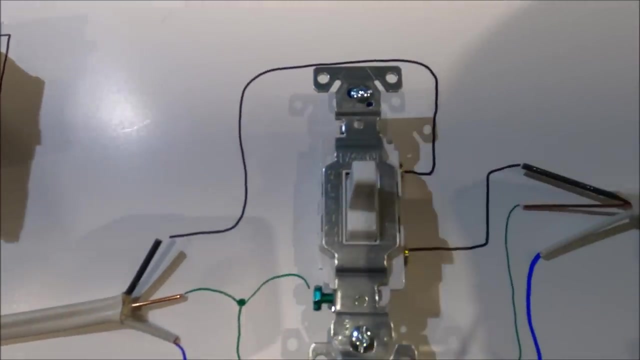 on just for good practice. We turned our breaker on. now, all of a sudden, the circuit's hot, so now it's flowing, or our power is flowing over to the first hot screw, You'll see that our switch is off. so this: these contacts aren't being made. but now, if we turn our switch on now, the electricity is. 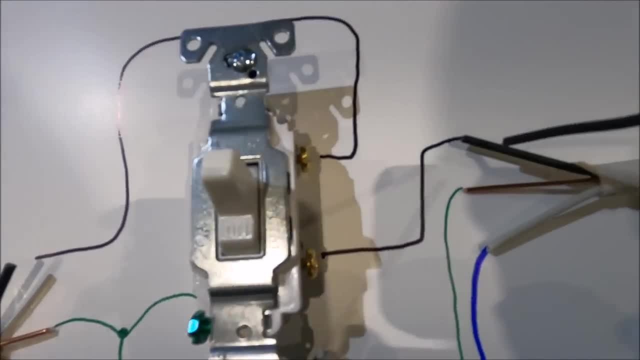 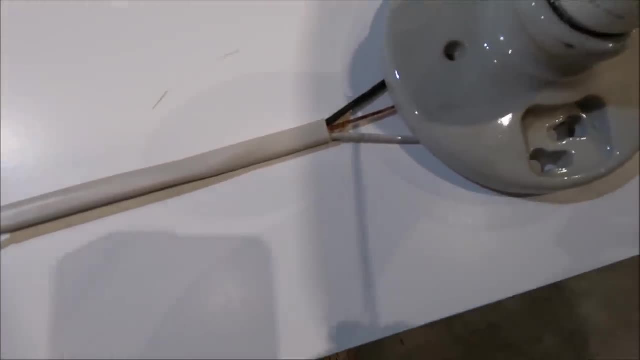 flowing through contacts made through the switch and it goes over to the black wire, comes over to your light fixture and then this light turns on and since this is on and completing a circuit, the power is also. electrons are also flowing back through to your panel box. 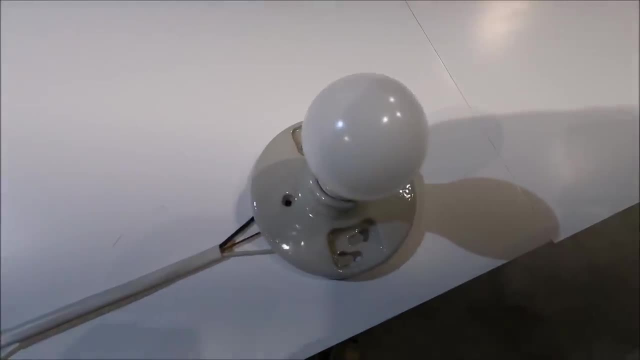 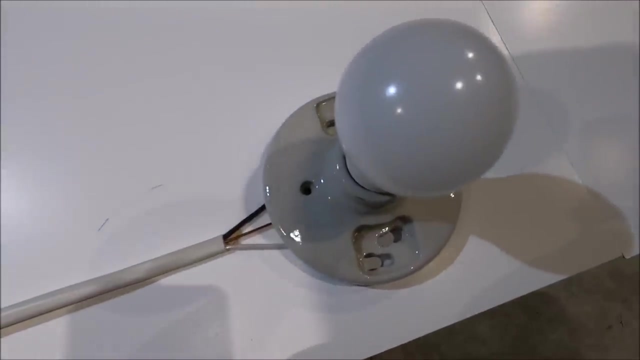 Completing the circuit. even though I have this little old timer light, this works with pretty much any light that you have and a lot of lights I've seen. they don't really have places to hook up the ground, so don't completely panic. If there isn't a place to hook up the ground, you just take. 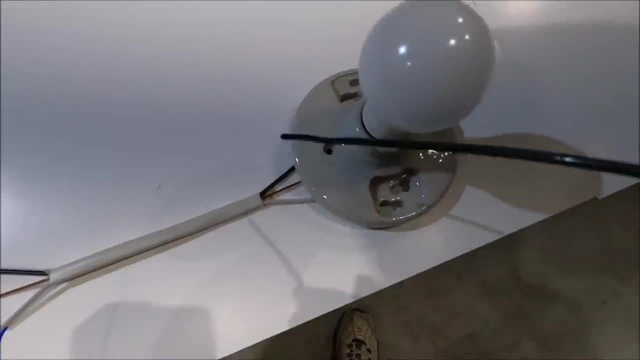 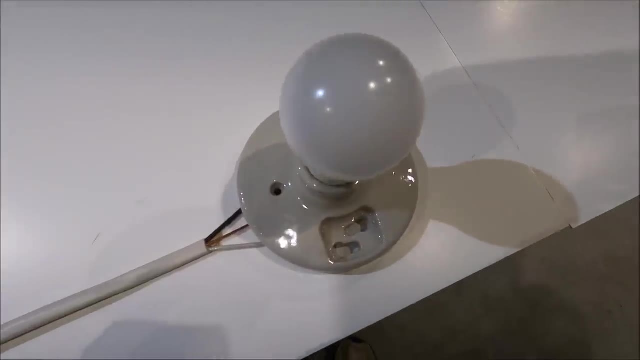 that ground wire and push it way up in the box out of the way. and if you have any questions, obviously contact a real electrician. I just play an electrician on YouTube. I know what I'm doing but I can't answer all the questions to everybody. 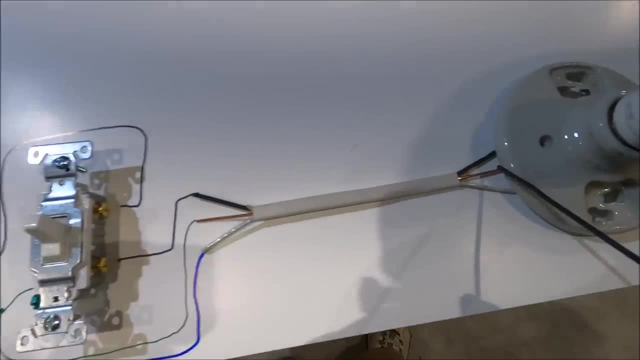 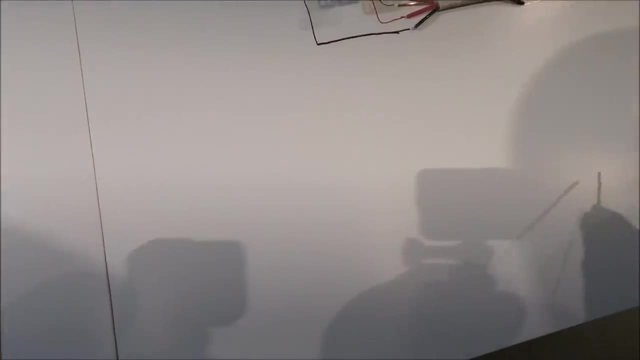 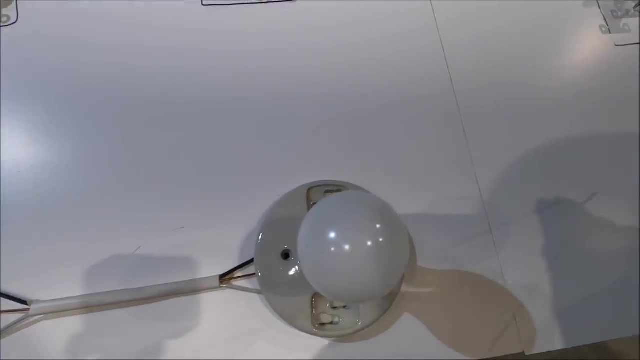 situation. as soon as this circuit is made here, you can put as many lights on here as you want, if these are wired correctly- which I'll show you how to do that when I'm actually wiring things up- and then it'll come, and then, as you wire these things up, the electricity will flow through. 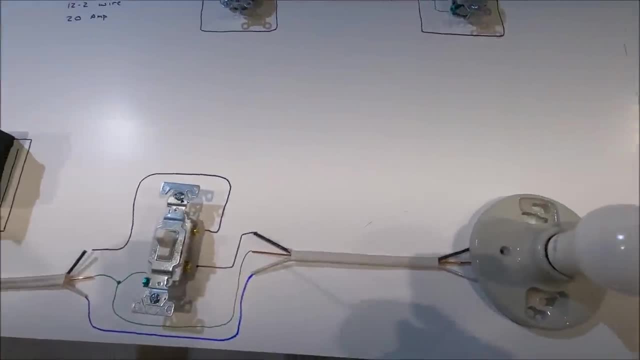 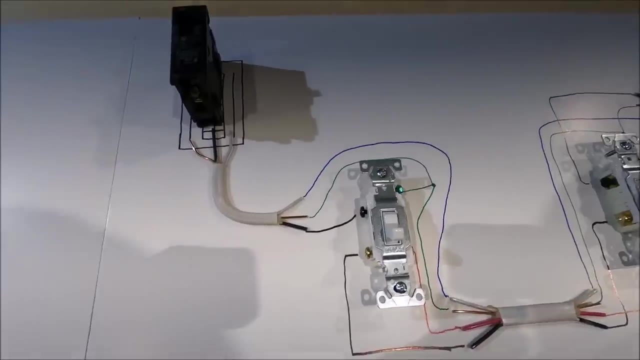 multiple lights and then end up completing the circuit. so really there's really nothing to be overwhelmed about. like just hooking these circuits up is actually pretty simple. so I can tell you people are pretty smart just by looking at you. and so we're going to move on to a little bit more. 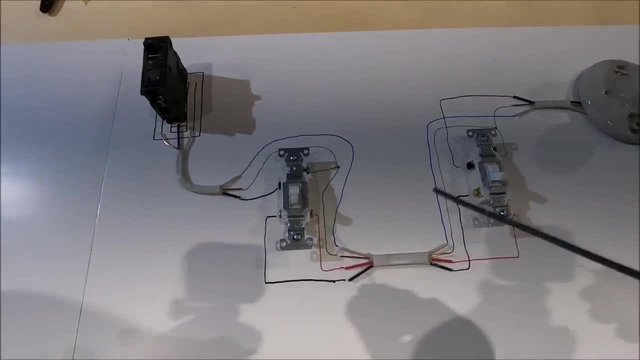 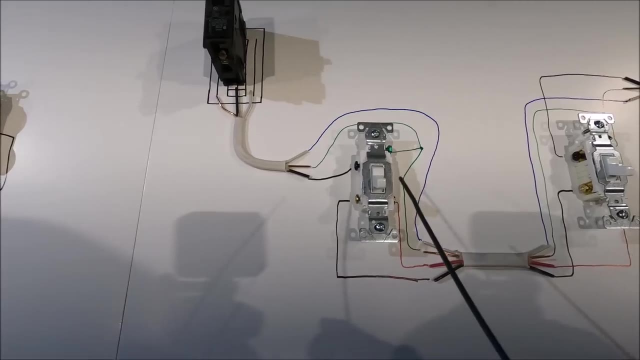 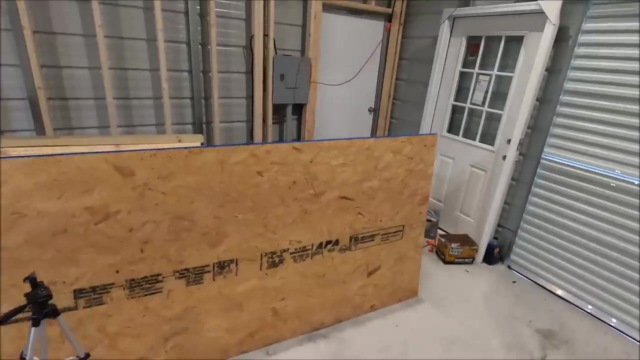 advanced circuit and this is a three-way circuit, and what this allows you to do is control a light from two different switches, and these are used for stairways or in large rooms or if you have two doorways. the reason I'm using them is because I have two doors, so what I want to be able to do 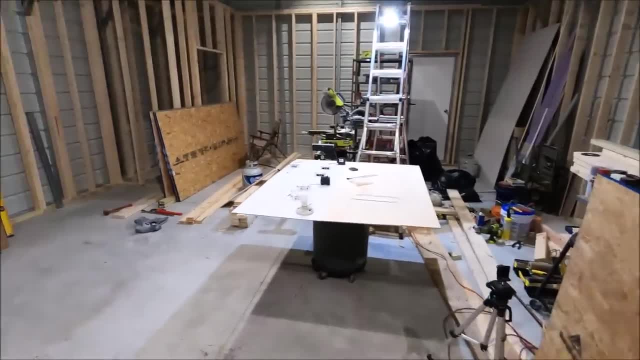 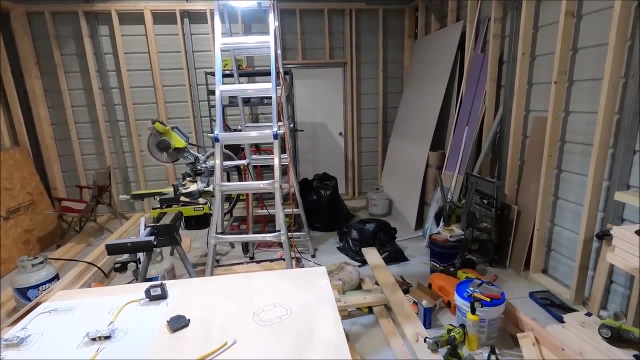 is: walk in this door or turn on the lights, grab a tool, do whatever I'm going to do in here and then be lazy and not walk out that door. I want to walk out the back door, and so what I can do is, as I leave, I flip the switch off over. 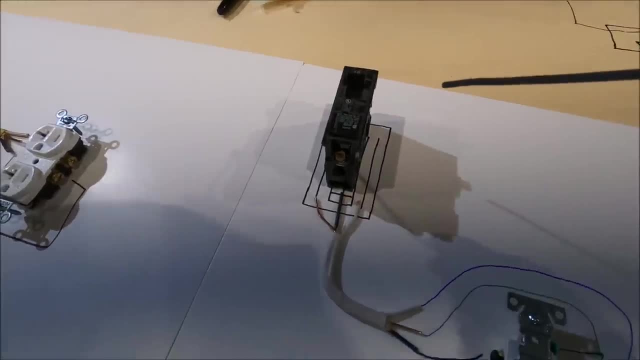 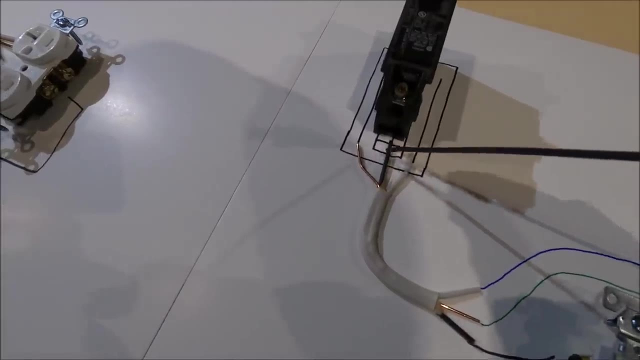 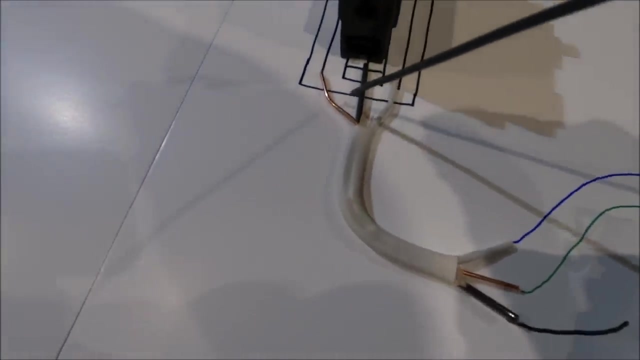 there and it still turns off all my lights. so same principle: here we have our panel box and we have our neutral and our ground hooked up to our bus bars and we have our breaker, and so same thing, the 14 gauge wire, the 14: 2 wire, is hooked up and it's pretty simple at first, comes over and it's. 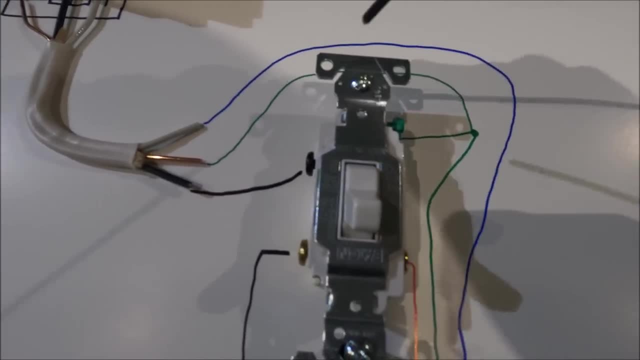 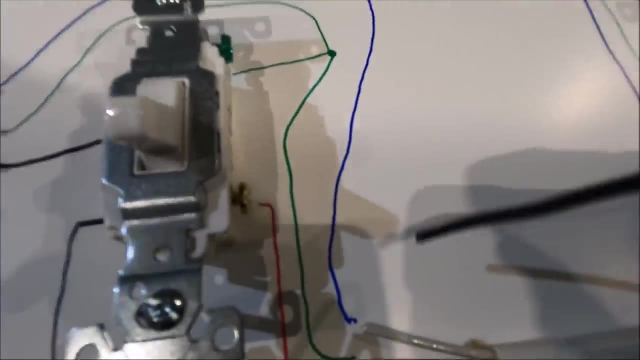 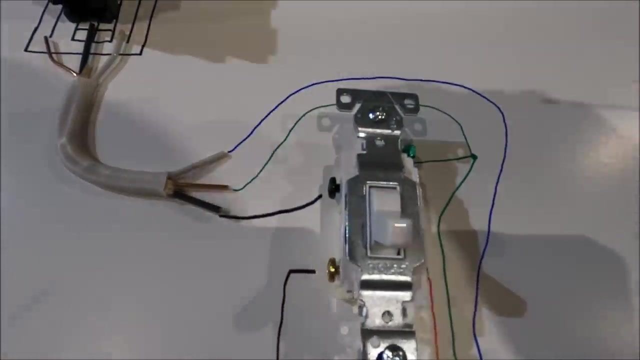 connected, just like we connected our other switch. we came up here, we hit a screw and we hooked up our ground and then we hooked up our neutral. this is where this gets a little bit trickier. with a three-way switch, your power comes in on the black screw and the way these switches work is as you. 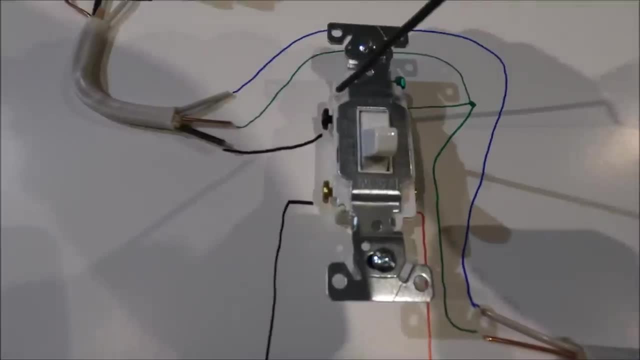 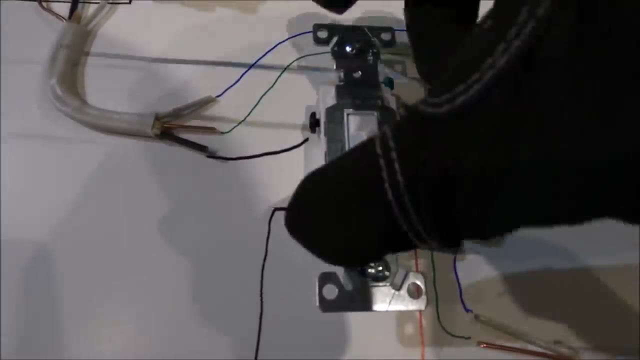 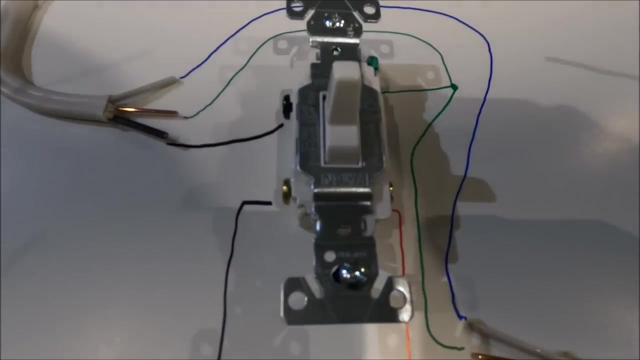 flip the switch up or down right down. right now you have it flipped down so say, like this screw would connect to this terminal. let's say we flip it up. this screw now conducts to this terminal. and why that's important is: let's say that the hot power is coming through the hot or the power is coming up to this screw. 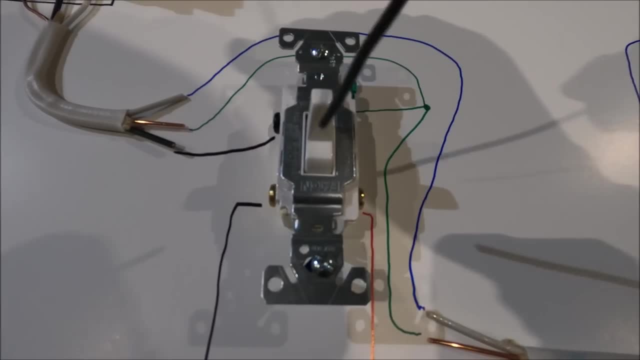 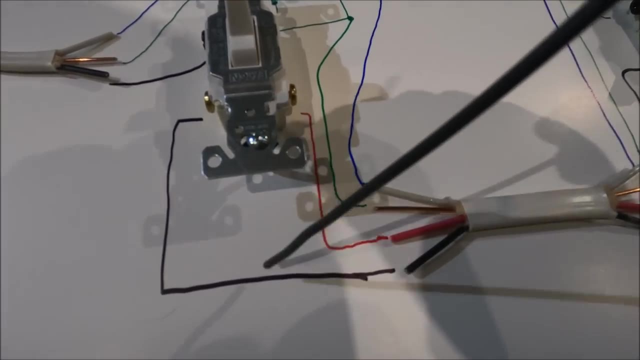 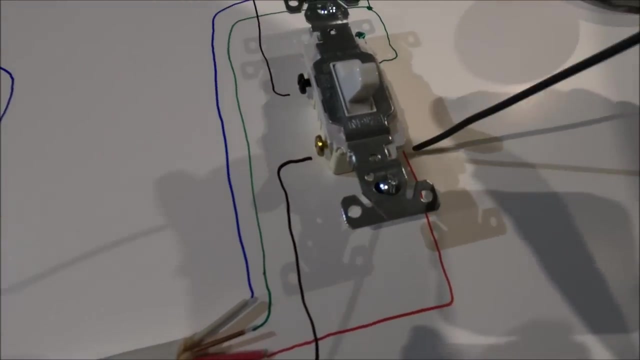 then let's say that it conducts across from this screw to this screw and then it goes into this red wire, and this red wire and this black wire are called traveler wires. so let's say that it goes across to this screw. now we follow the red across, we come up here. now, look, our switch is down. so let's say: 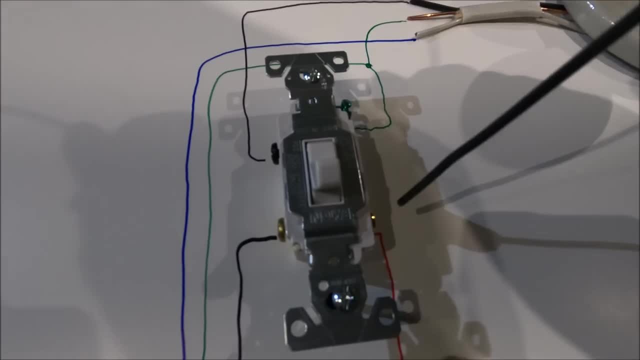 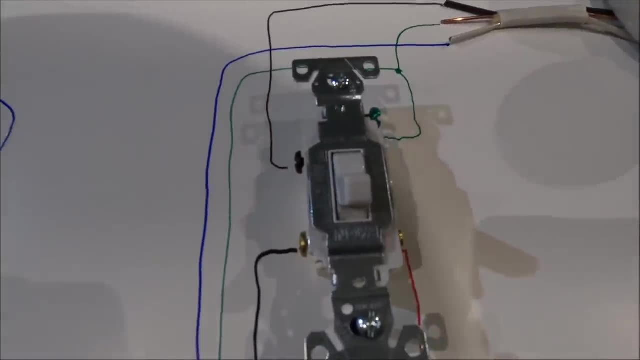 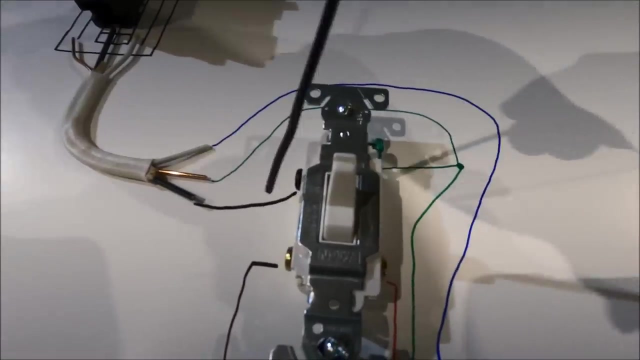 that this black screw is connected to this screw. well, now there's no way to conduct across, to make it to complete the circuit for the light, and this is how three-way switches work. right now you can have power up to this switch because somewhere power is coming through up to this switch and this is. 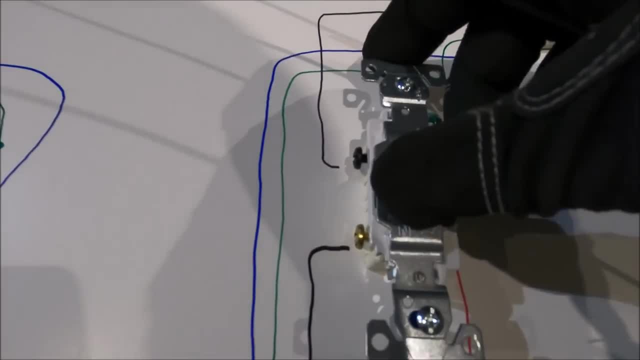 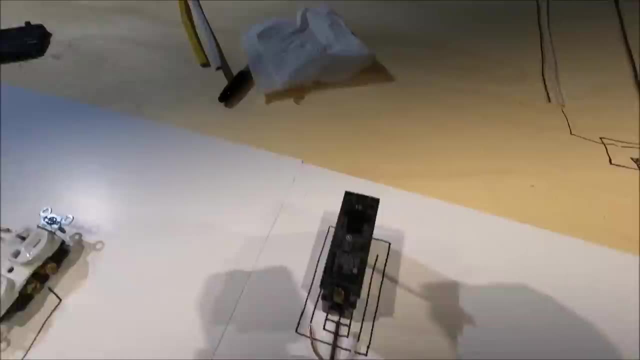 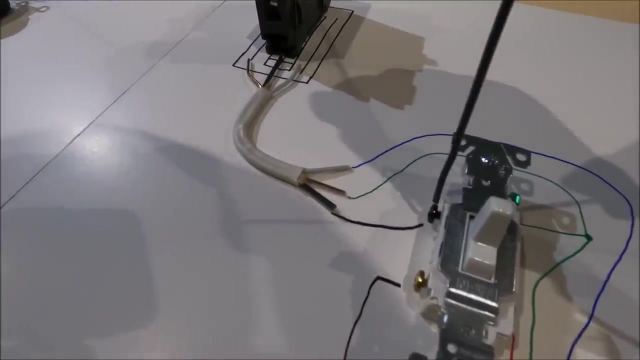 where it's going to break. so say that i flip this switch up now. let's follow the path of the power. i'm getting really bad shadows here. so now we have the black wire coming over to the black screw, comes across to the red, to this screw here. 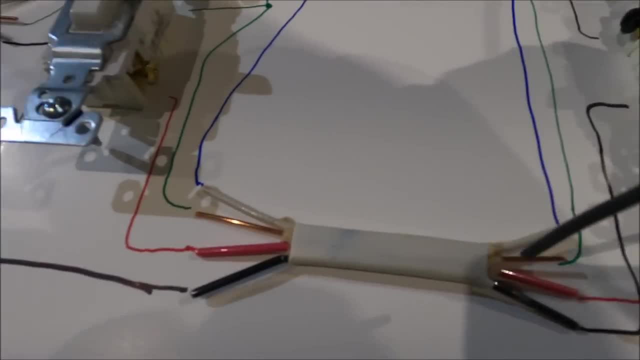 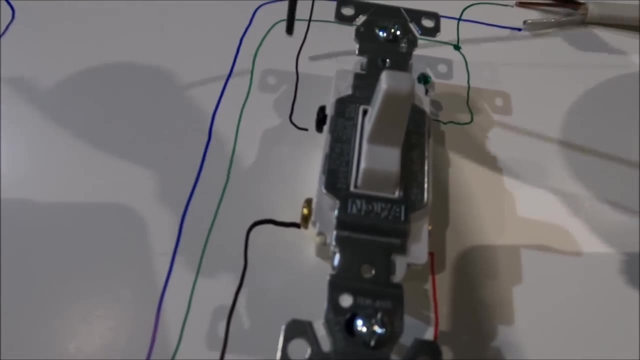 and then we have the black wire coming over to the black screw and then we have the black wire, connected to the red wire, comes across, hits the red wire. now it comes over to this terminal here, the screw here. now it conducts across. and look what it does: it hits our light power hits. 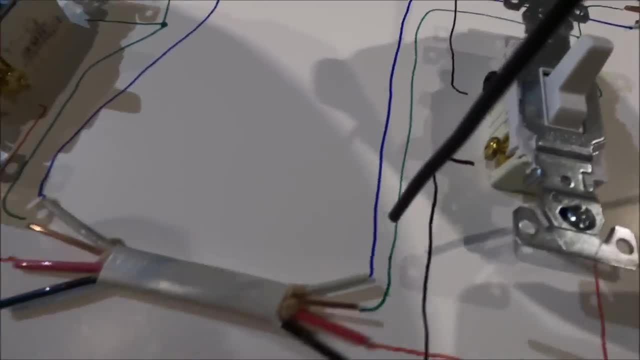 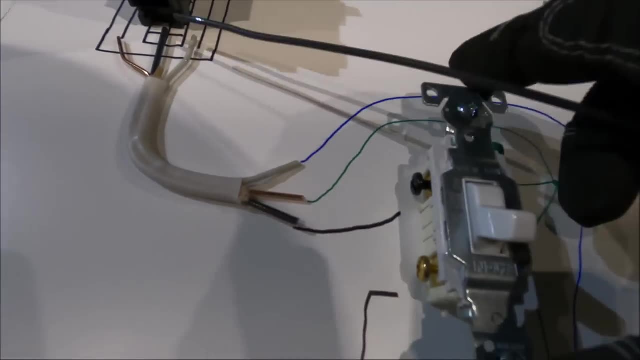 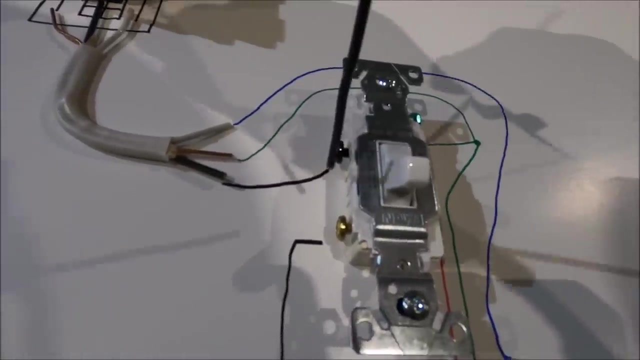 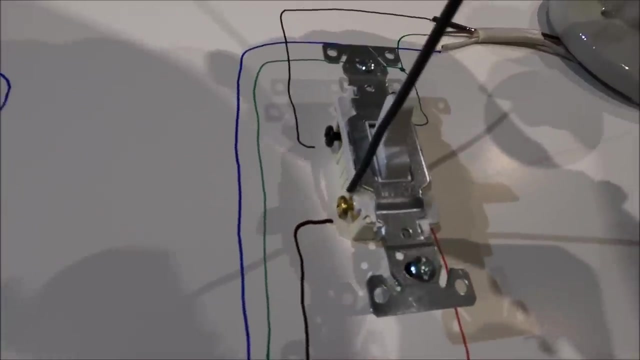 our light goes back through the neutral wire. it goes back around, back to our panel blocks. we've completed a circuit. now let's flip this switch off. let's see what it does. now black wire comes across, hits this screw here, comes to this screw. now we follow the black wire around. except for this, conducted this way. 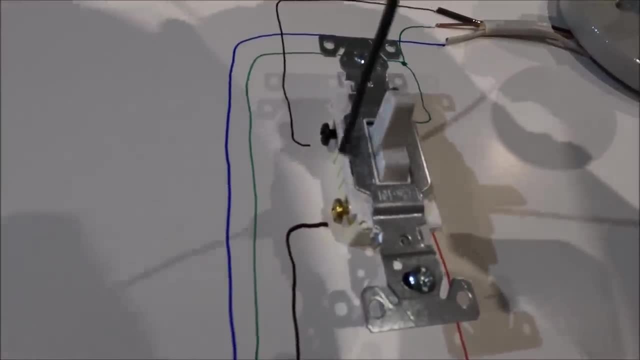 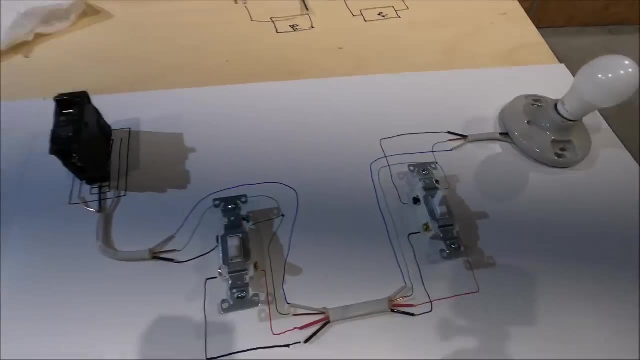 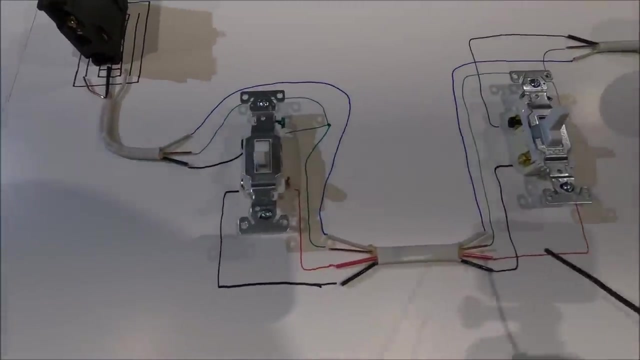 without switch being up. now we have no conduction through this screw to this screw, which means the power won't make it to the light. and that's how three-way circuits work. is these two switches kind of work together to break the circuit through these traveler wires? and that's why you need a 14. 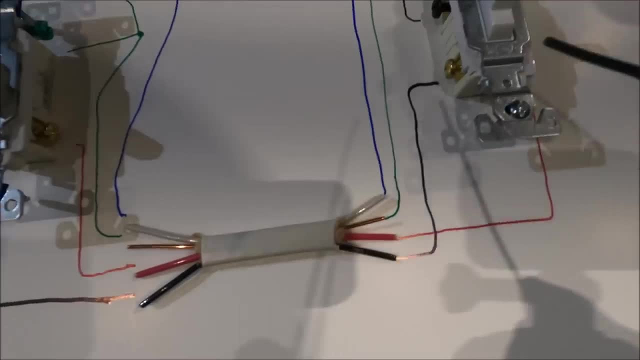 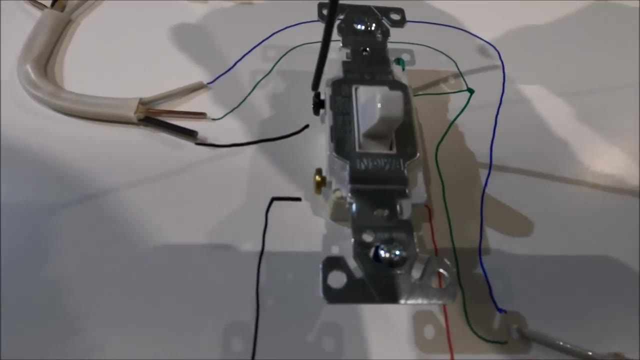 three wire to break the circuit through these traveler wires, and that's why you need a 14 three wire, because you need this extra wire for traveler wires. so when you wire this circuit, you're going to wire up the switch just like normal, just go up to your black screw wherever the power is coming in. 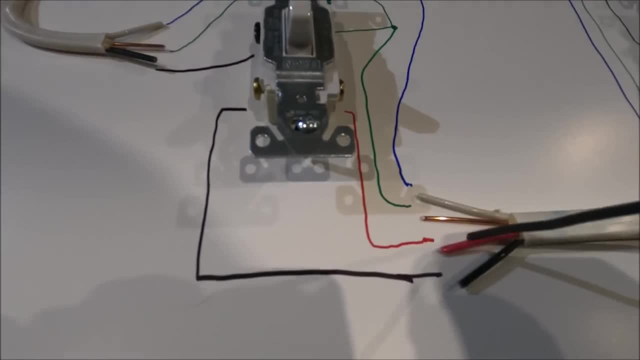 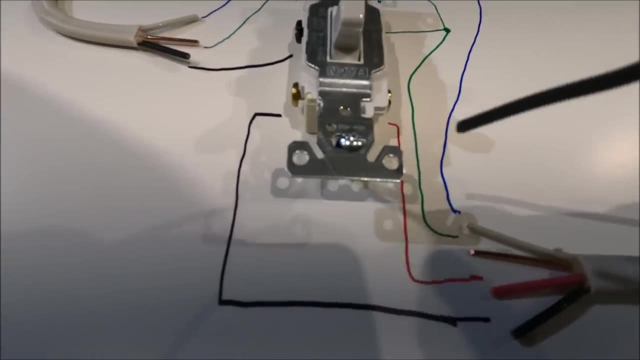 at, and then you're going to take the black wire and the red wire and hook them up to whatever terminal. whatever screw you want, doesn't even matter. but when you come over to the other side, be consistent. if you hook the red screw up, you're going to get the black wire in there, so that way. you don't have to三- ****, you have to move your wire across yourself and on your is préc cream over to where your alba is reflecting the signal this Smith and appearance is correct to conduct, to connect even a tangio. I'm comenzar to show you just grain our final design before I'll just have the black work and this Сегодня the white wire. 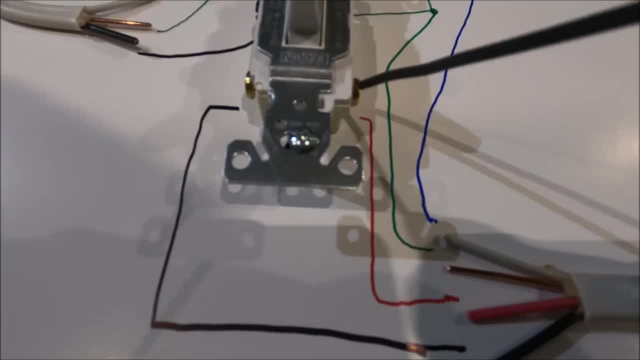 look at what's built up blocking this once. connect to the plug. so when you have the在vent la rose wall I'll show you some other up. or if you hook the red wire up to the screw on the right, do the same thing here and hook the. 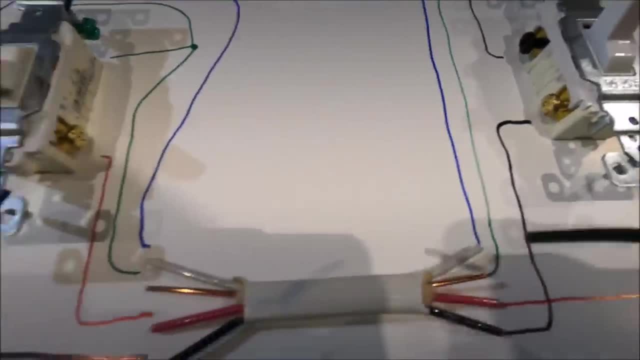 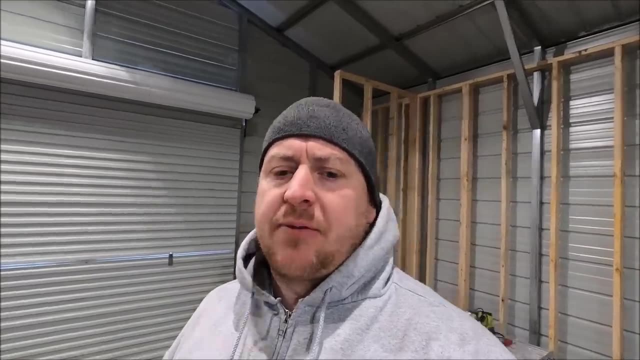 the red wire up to the screw on the right and same thing with the black. you just want to be consistent. so these circuits are pretty basic. throughout your house there's different outlets and stuff you can use with the gfcis and i'll wire those in later and explain a little bit more. 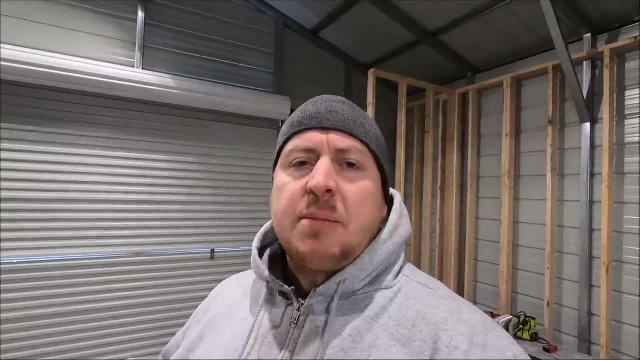 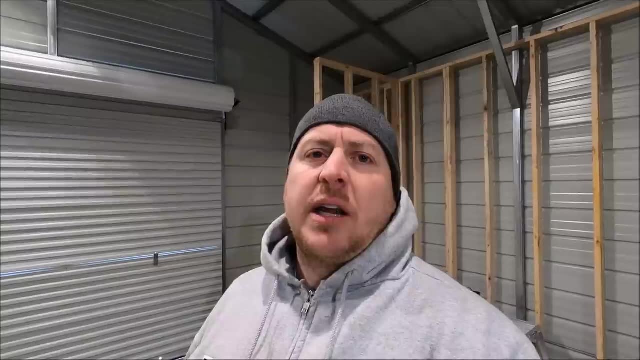 about what they are, but i just want to do a video on some of the basic wiring. i have a bunch of friends and stuff that you know. i always do their wiring or i'm trying to teach them how to do wiring and they're interested in learning, but they just need some, some way to get started. so 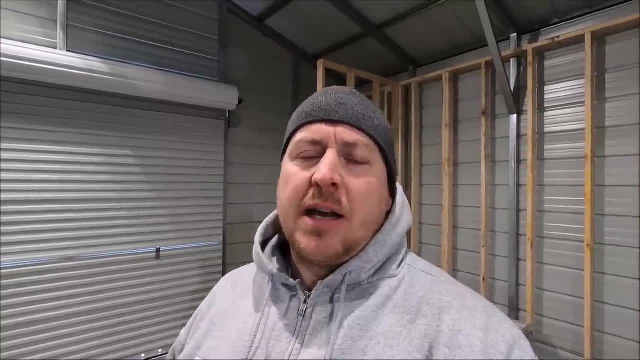 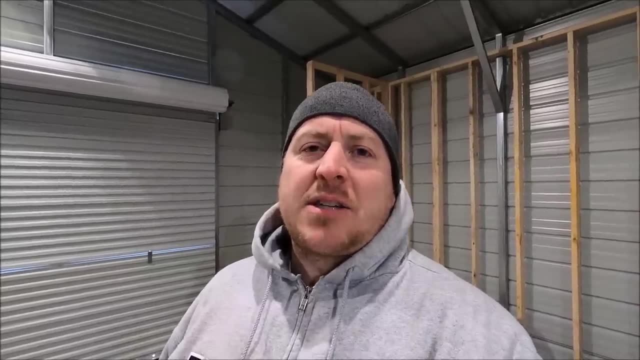 i hope this helped you out. i really enjoy teaching people how to do things. i've got comments that they're like: oh you know, you do a good job explaining stuff. i try. i do have a master's degree in education, but i don't teach because i think the education system is a little wrecked. 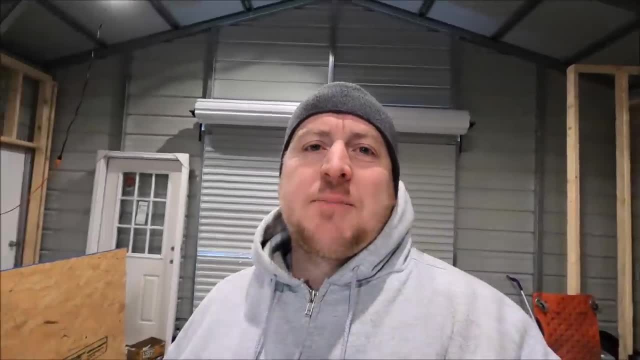 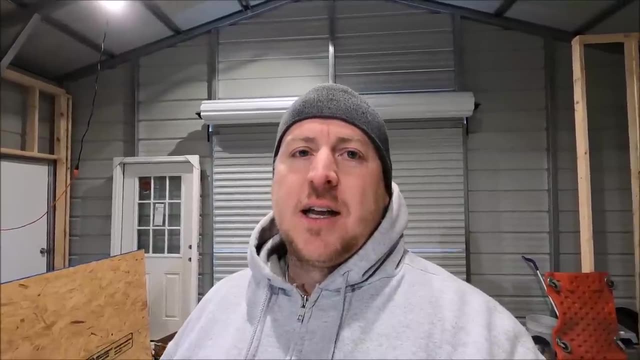 right now. hopefully they'll fix it, but i do enjoy teaching people. so if there's anything that you'd like to learn- i mean i don't know everything, but i certainly- if you have any questions about these circuits, please put them in the comments and i'll try to answer them. so i'm going to be. 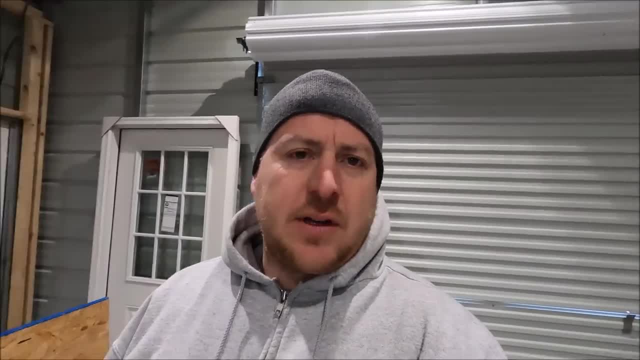 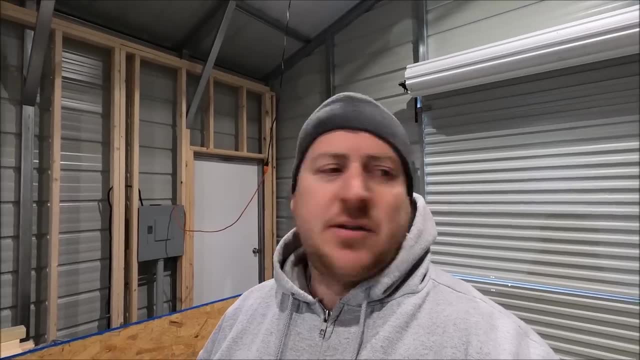 buying lumber here in a couple days, now that my friends finished up with their jeep, tried to get things a little bit more organized in here and get all my toys in my toy box. i don't know, this place is really hard to work in right now and i'll work on finishing up a couple small walls. 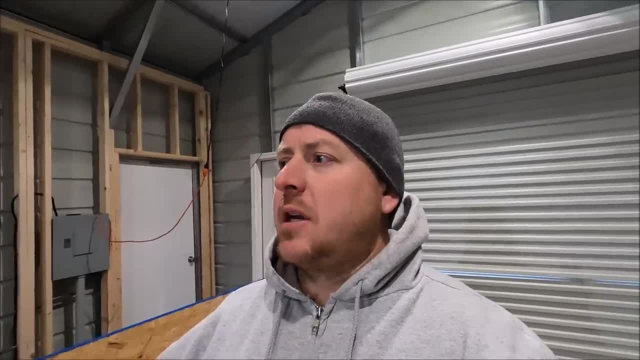 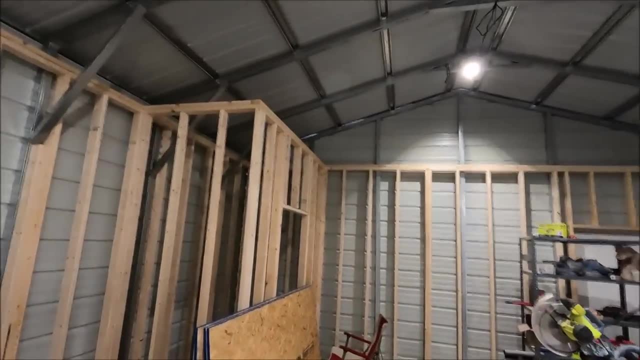 that you've basically already seen how they get framed up. so i'm going to hurry and throw up a few walls and then i'm going to put those beams on the top, and they're not going to be very high, they're only going to be. i think i'm going to do two by eights, just because the span is going to. 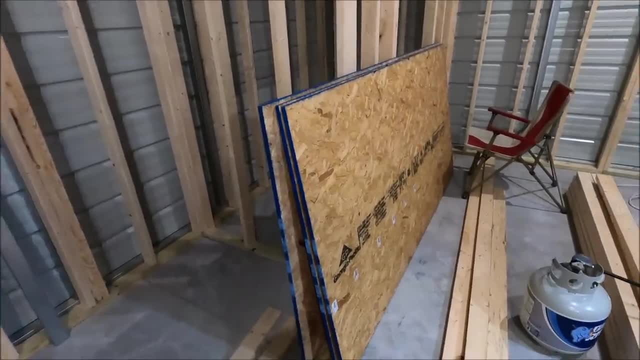 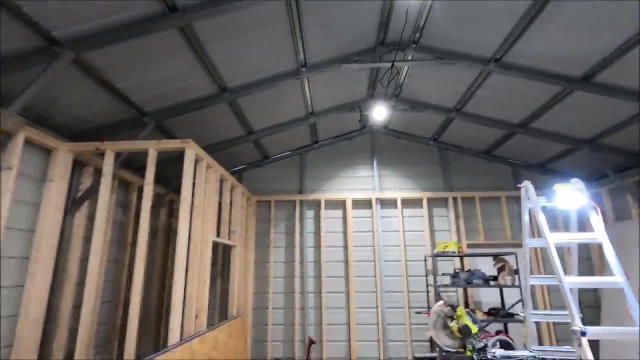 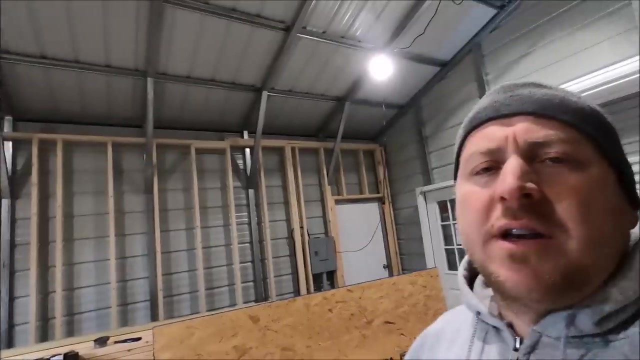 be very long and i'm going to also build them out of some plywood and i'll show you how i'm going to put those together and then after that i'm going to span- i think it's going to be two by eights across, because i can't seem to find the number one, yellow pine. i don't know if anybody out there-